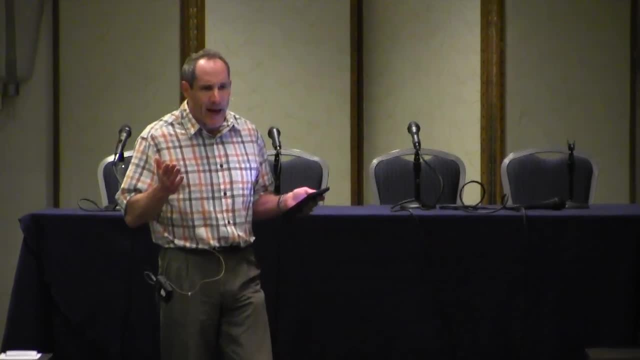 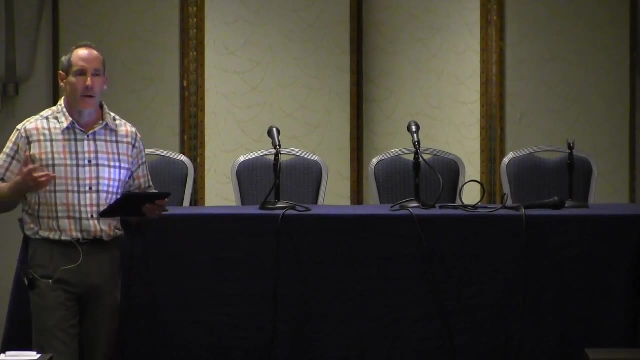 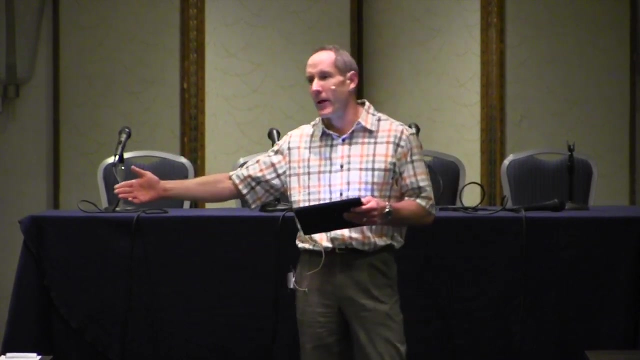 And when I thought about this I thought how many diagnoses are just purely clinical? Oftentimes, of course, we generate a differential diagnosis And we start thinking, gee, maybe it's appendicitis. And then almost invariably, you're getting the cat skin, because surgeons don't operate without 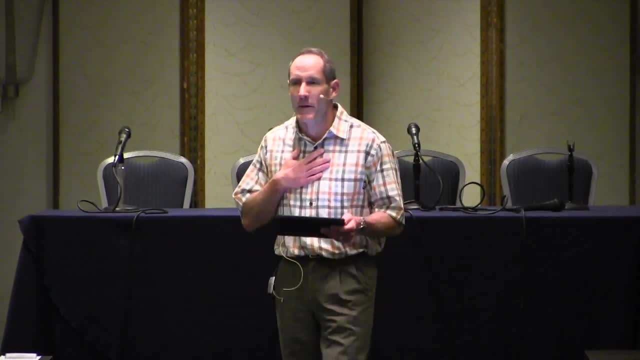 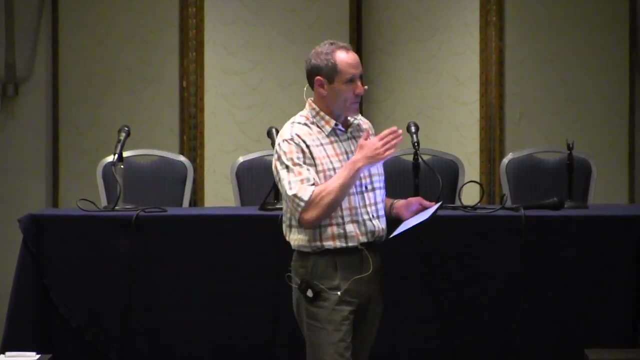 a cat skin anymore, Or even if it's, you know, I think it might be pneumonia And you're trying to get the x-ray to confirm pneumonia. This is one for which there really is no confirmatory test. It's a purely clinical diagnosis, And I think most of us have learned over time what the five 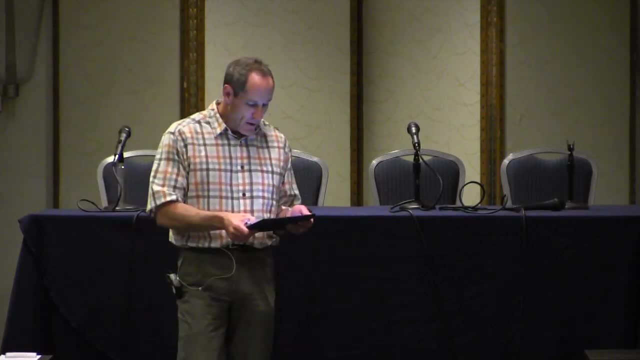 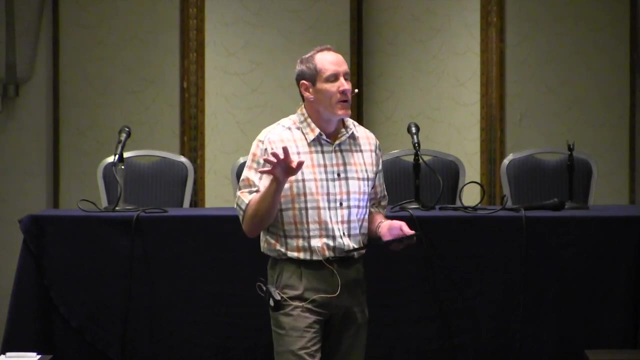 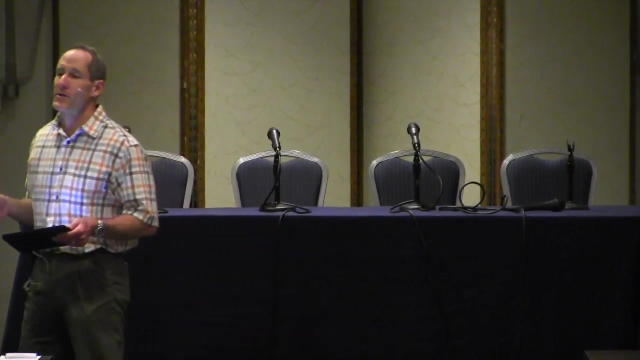 cardinal signs and symptoms are, And so I'll repeat them here. You're supposed to have four or five of these, And generally it's in the setting of five days of usually unrelenting fever, So sometimes it can be intermittent. And of course, if you catch the kid on day three, you don't have the benefit of days four and five. And you have to start thinking about this- the longer that the fever is going on, But usually it's five days of fever, And then you get, actually without me even saying it. So tell me what you get with Kawasaki disease. What are some of the things you're looking for? Lymphadenopathy. Lymphadenopathy- So usually we call it mucocutaneous lymph node syndrome. Lymphadenopathy: supposedly it's cervical lymph nodes Supposed to be 1.5 centimeters or greater. That's what you're looking for. So we got lymphadenopathy. What else? 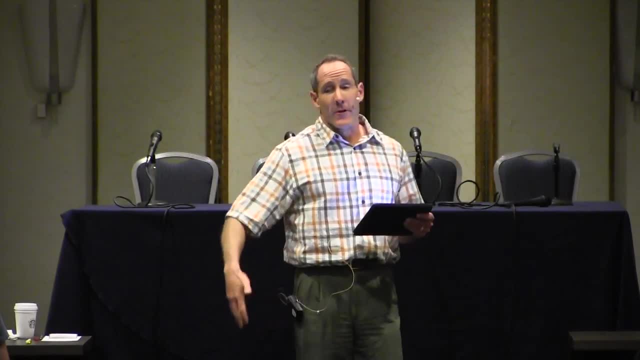 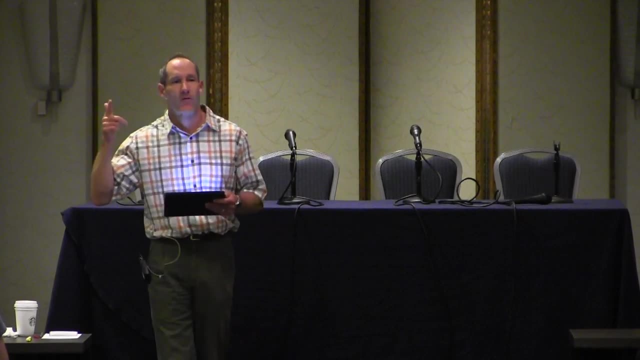 Rash Rash, So often a diffuse rash, But of course rash is a disease. Rashes in kids are generally diffused and can look like anything, So we got lymph nodes rash. What else Extermine edema? 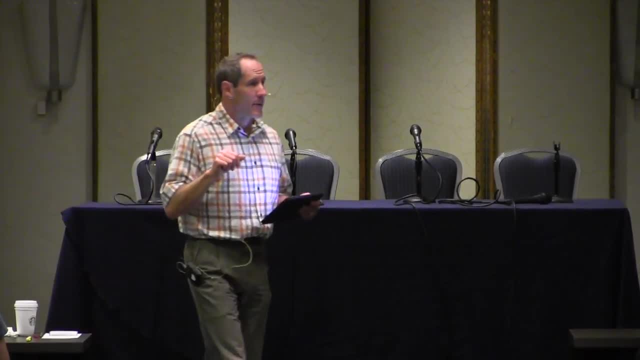 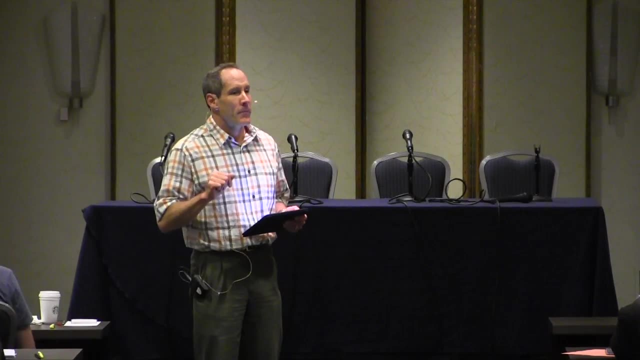 Extermine edema. So you get hands, feet Look for that And eventually you get desquamation once the edema is going on for long enough. We're missing two Conjunctivitis: Conjunctivitis. 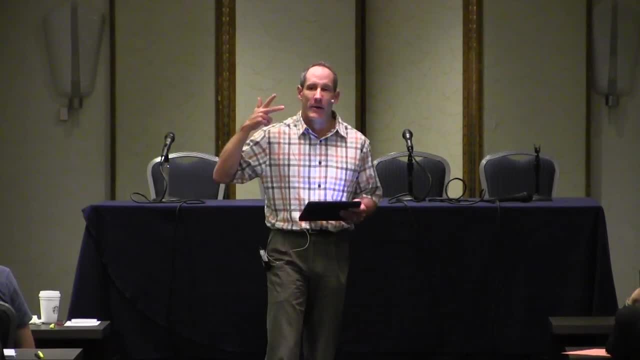 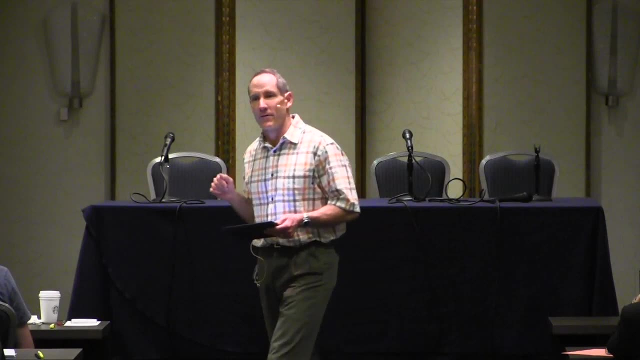 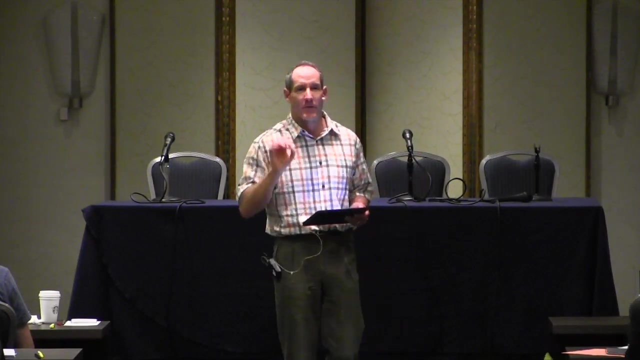 So rash fever and conjunctivitis should really be starting to trigger the thought of Kawasaki disease. And then what else? And it sort of goes along with conjunctivitis, It's the oral findings. So you can get the cracked lips, You can get swollen lips, You can get the strawberry tongue. 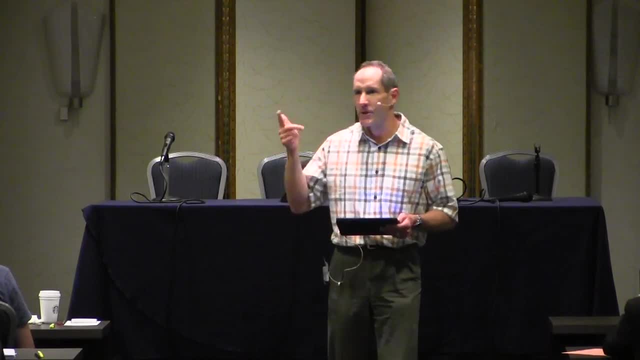 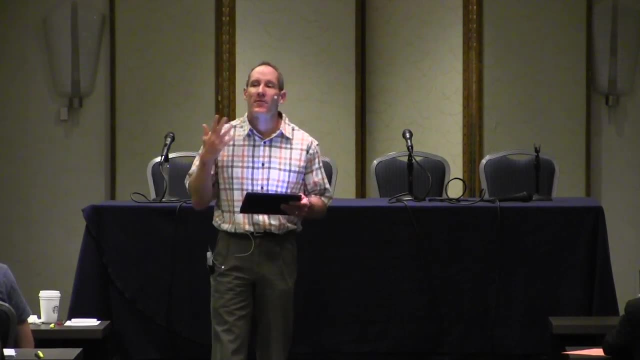 So those are the things that you're starting to look for. So really, it's kind of rash, fever, conjunctivitis And then anything going on with the lips, the fingers, Start thinking Kawasaki disease, The main complications of Kawasaki's that we worry about. Generally it's a self-limited disease. People are not dropping dead of this. It's about a 1% mortality rate, though, if it's undiagnosed, untreated. What's the most feared complication of Kawasaki Cardiac? So you can get a myocarditis and you can get coronary artery aneurysms And that's hopefully what you're trying to prevent. The treatment is IVIG And, as best I understand, if you catch it any time, within about the first 10 days of illness. and you start treating with IVIG, then the outcomes are better than later on. So it's not the first five days of illness. It's not the first seven days of illness. You've got a little bit of window there And, as you can imagine, you see these kids on day three. 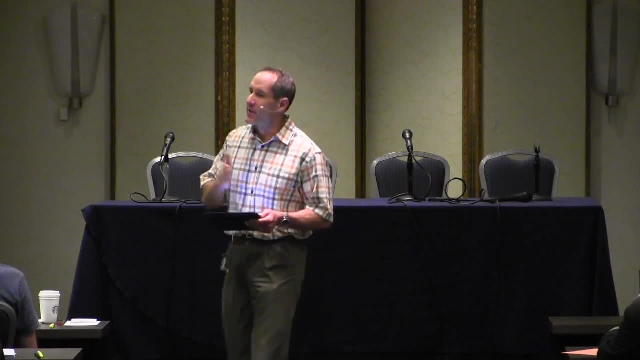 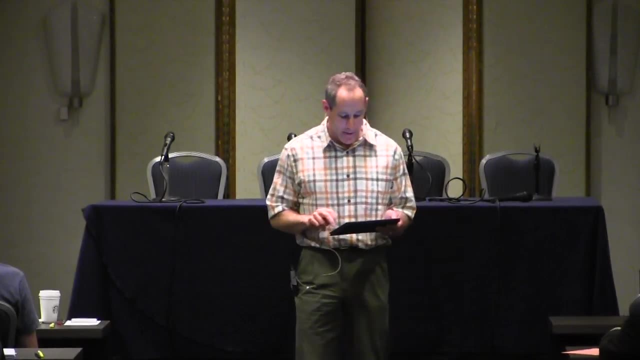 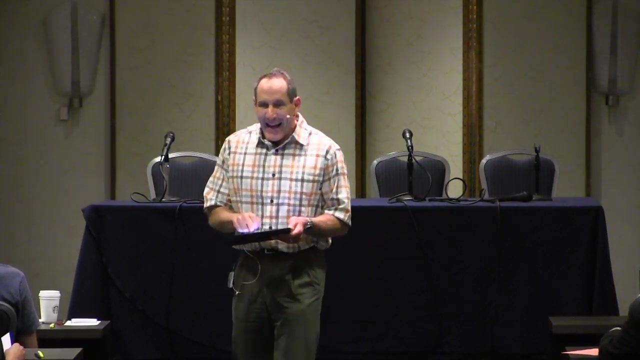 You might not be thinking about this, Certainly by day five, day six, unrelenting fever And the more of those other items that you find it should be starting to show up in your brain. As I said, no medication. There are no laboratory studies to confirm Kawasaki. 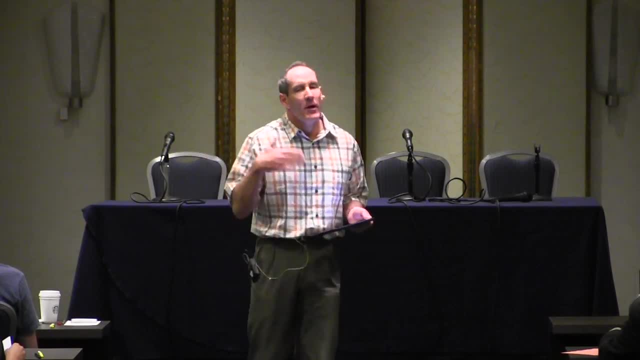 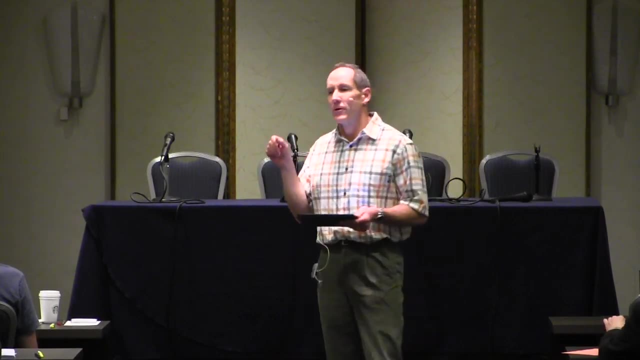 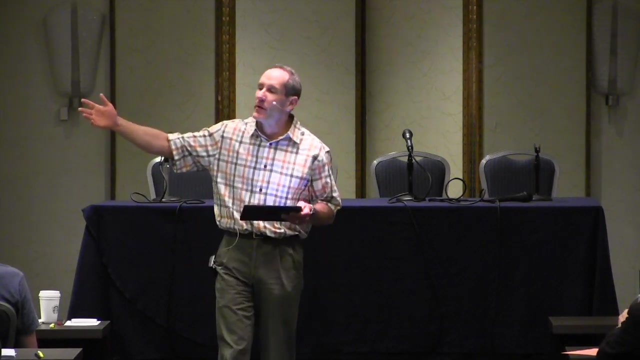 And because it's a systemic inflammatory disease, you can find other signs of inflammation, So you can get pyuria, which is usually due to essentially urethritis. So if you start saying, oh, the kid's got a fever, but hey, there are 15 white cells in the urine. 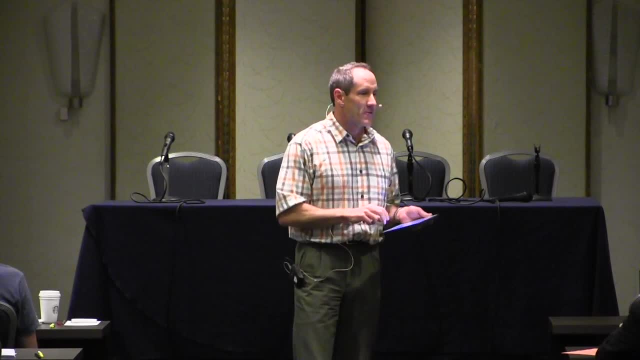 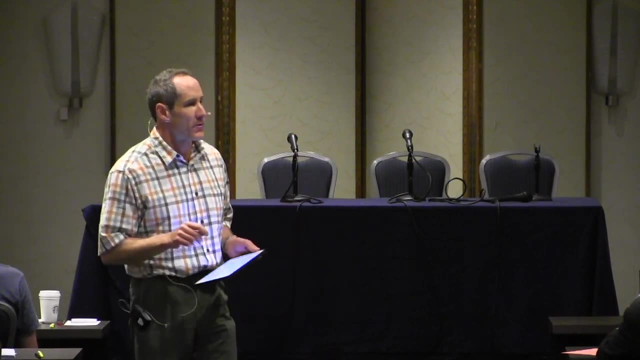 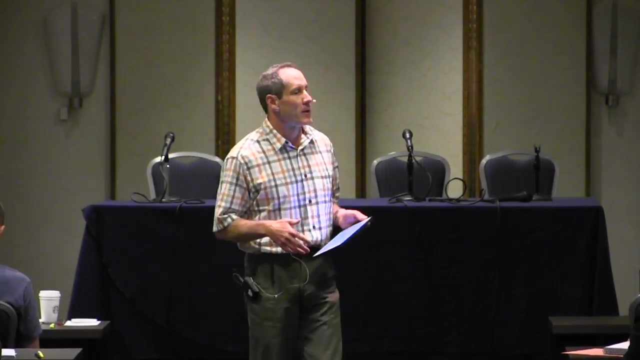 It must be a UTI. If you've got some of those other features, think again. Other comments, thoughts, questions about Kawasaki, Because I'm just going to keep moving. Okay, The next one is not my favorite. So, as much as I like Kawasaki because it's clinical and we're going to see it, the next one is not so much. 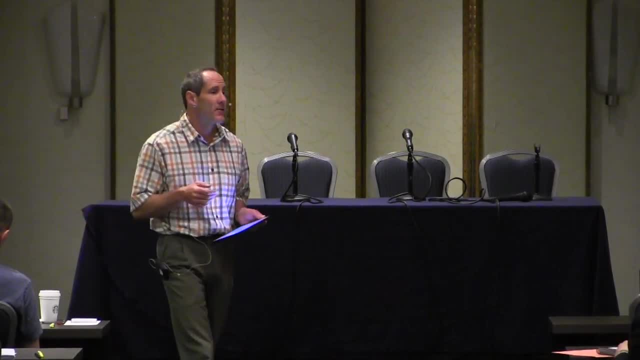 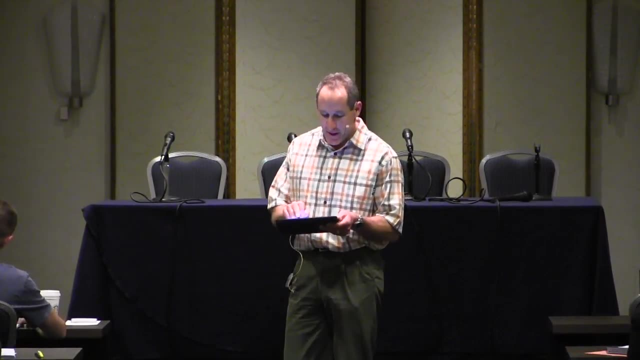 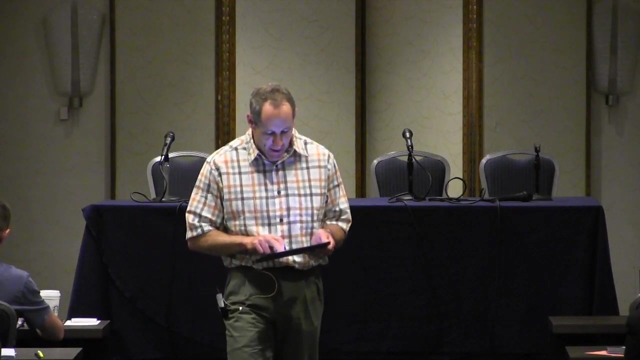 So it's myocarditis, And we already mentioned Kawasaki is one of those things that can cause myocarditis, But ultimately, myocarditis is a fairly uncommon disease. Oh, I'm sorry, I did want to say one more thing about Kawasaki's. 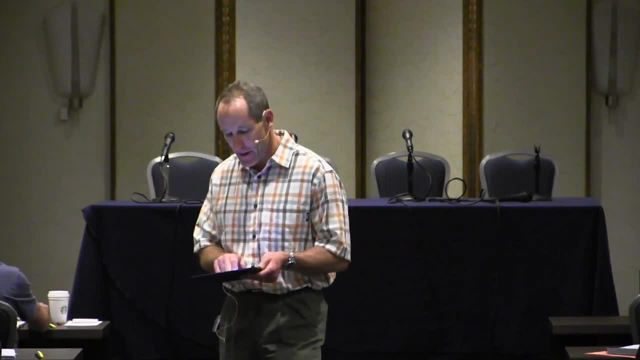 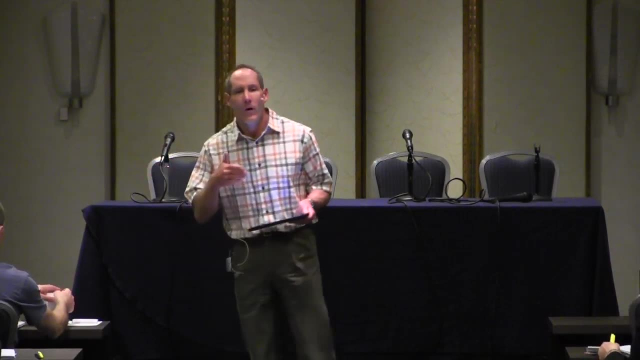 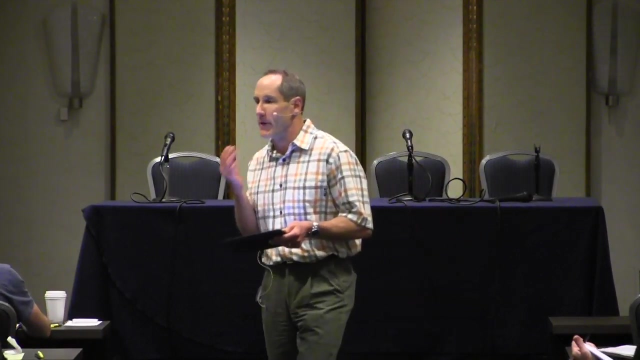 That, depending on your age of presentation- and I guess I should point out some of the abstracts, for hopefully most people have their books now- There are a little bit of differences. So older kids: there's a little table in your graph. Older kids tend to present with a cervical lymphadenopathy more than the younger kids. 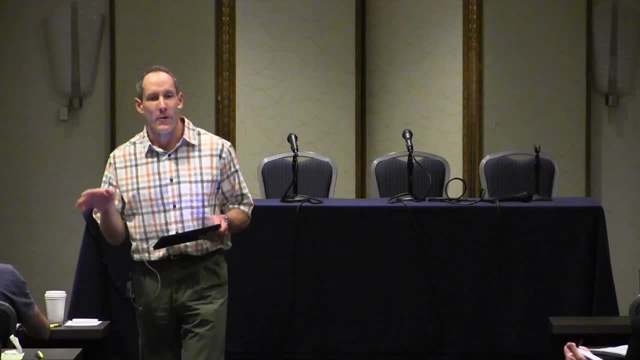 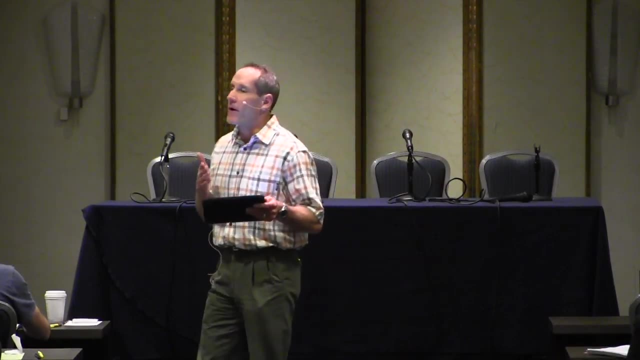 Older kids present more with the rash and the conjunctivitis. So there's a couple studies here, abstracts two and three, And just be aware that there are some age differences, But ultimately many of the kids will have all those elements. 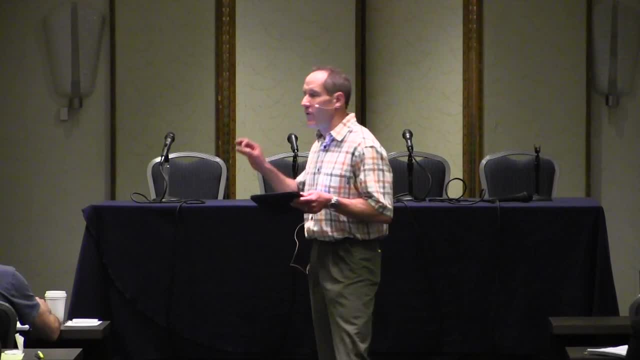 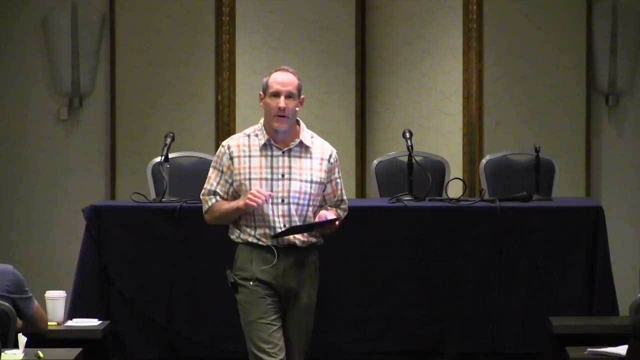 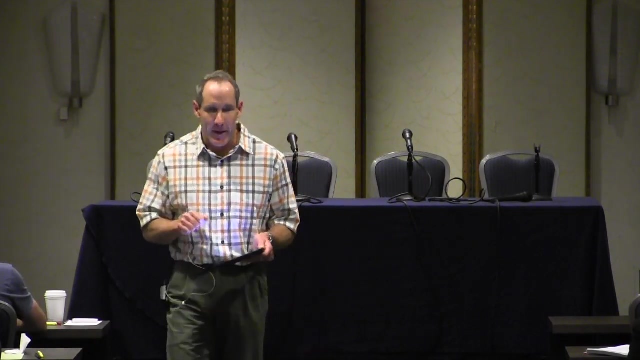 But a lot of them do not, And you don't need four, You don't need five to necessarily make the diagnosis. You can start thinking about it and at least discussing with your consultants when you start having more than a couple. Myocarditis is a presentation of generally congestive heart failure in kids. 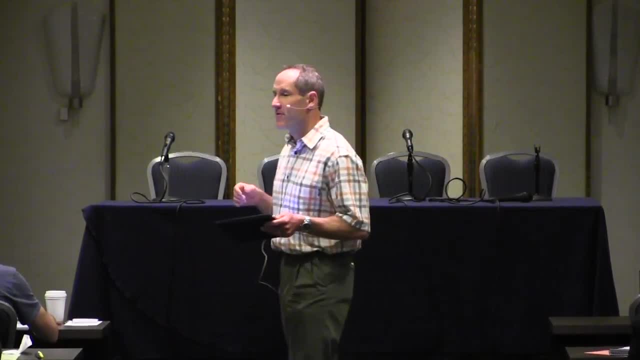 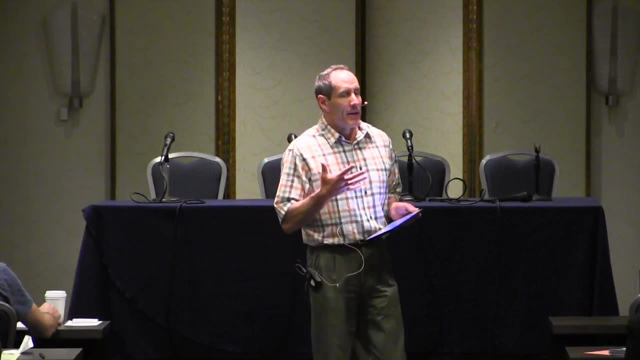 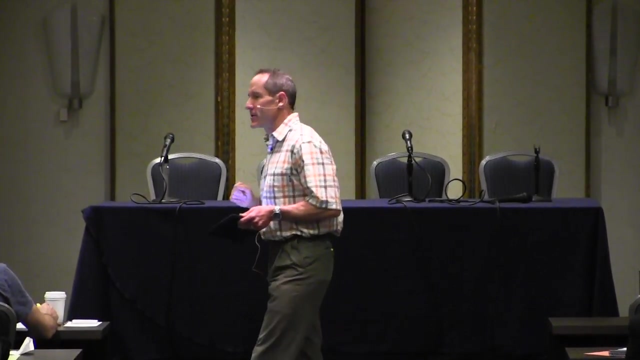 Adults tend to have a more chronic subacute myocarditis. when we see them, Kids tend to present more fulminantly or acutely, And when you start thinking about congestive heart failure in kids is when you start coming up with a presentation of myocarditis. 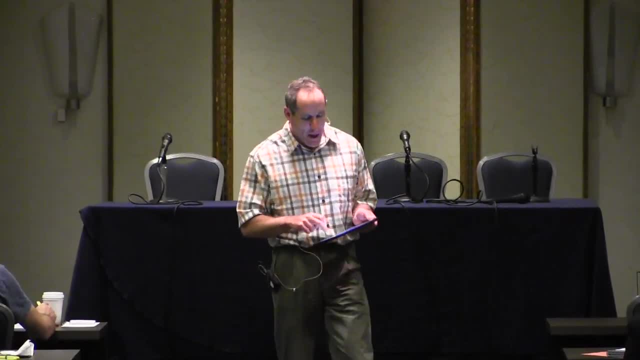 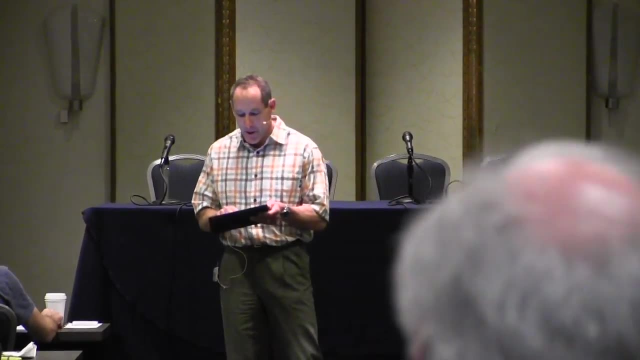 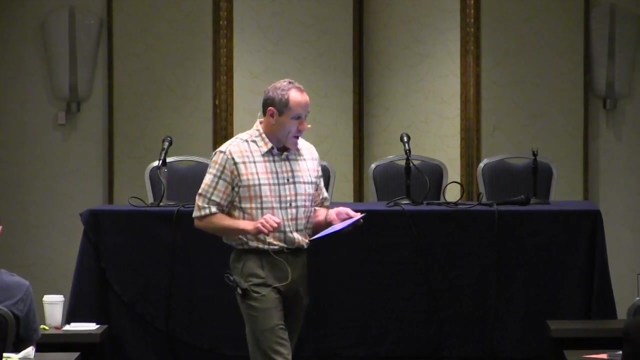 Which, as you can imagine, is not common. Often it's a respiratory presentation, So you'll get dyspnea at rest, exercise intolerance, tachypnea. Physical exam will often have hepatomegaly, But ultimately you don't necessarily think of it when you're seeing kids who present with chest pain. 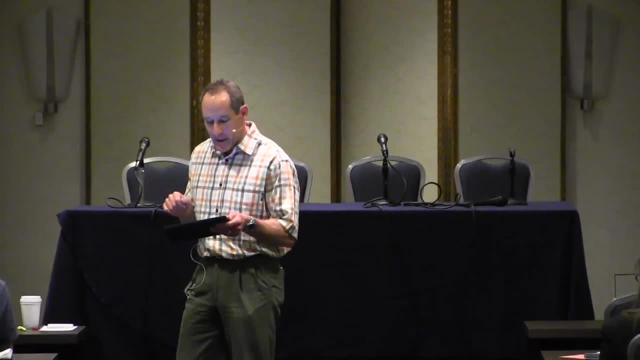 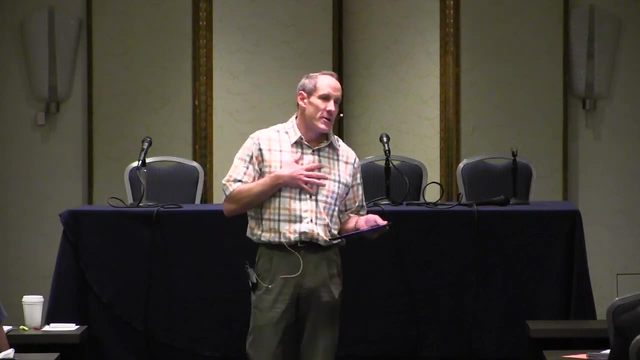 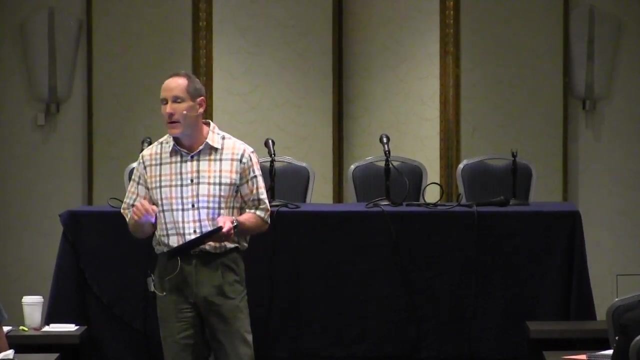 So abstract four talks about cardiac disease in pediatric patients presenting to a pediatric ED with chest pain. In adults, people walk in with chest pain And I think the first thing most of us are thinking about is: is this an MI? Is this an ACS of some flavor or other? In kids it's essentially fear not. In this study, of 4,300 kids, 0.6% had ultimately a cardiac diagnosis. So under 1% of kids who present to you with chest pain are going to have a cardiac diagnosis. 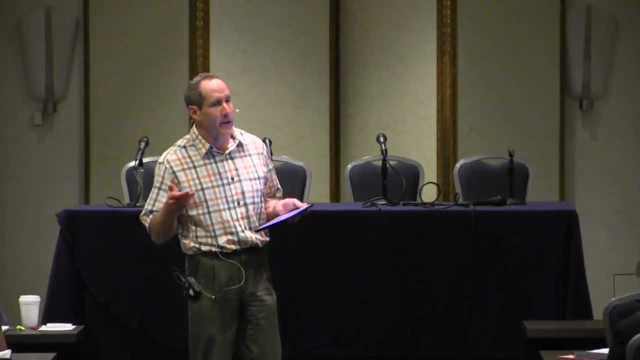 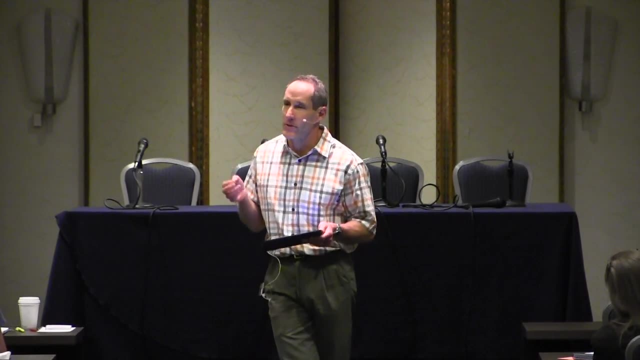 And of the cardiac diagnoses that they had. it wasn't like these kids were presenting with MI. There were a couple, But it was mostly dysrhythmias, usually an SVT or pericardial disease- acute pericarditis. So certainly an SVT is going to be a little easier to spot than an MI in a 7-year-old. The latter rarely happens, But for the most part chest pain in kids, you don't have to worry so much about Cardiac etiology. 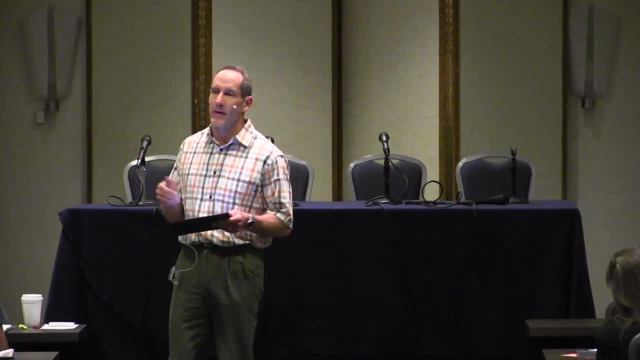 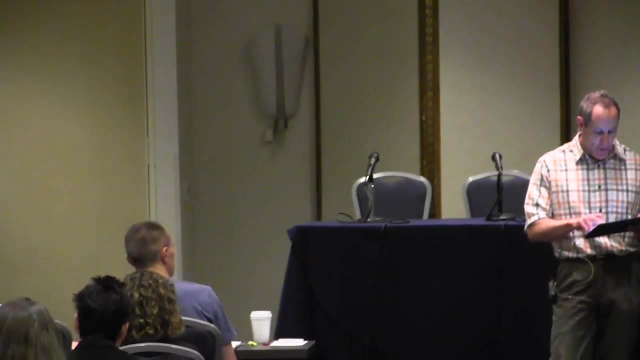 Obviously, you're doing your history, You're doing your physical. You can easily get an EKG if you're so inclined. But one of these next papers- Metroponin value in kids. I'll be skipping around a little bit here. 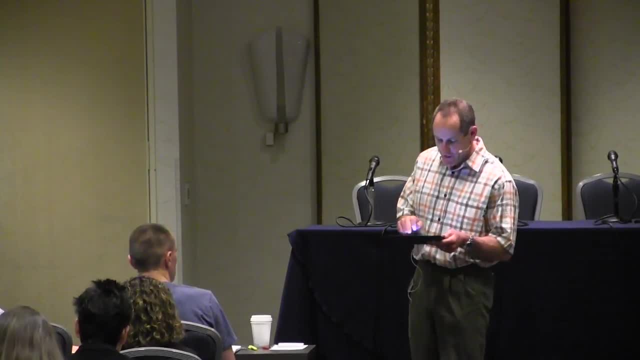 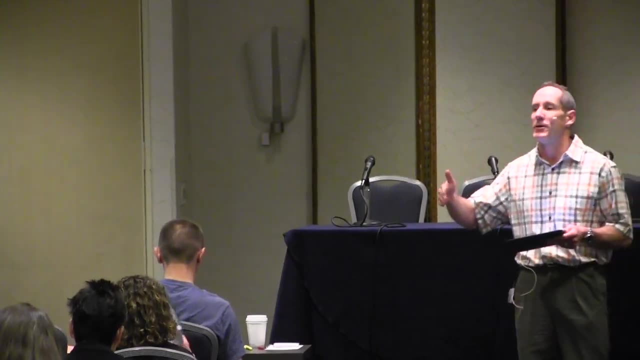 I think that is abstract number seven, Since we're talking about chest pain In adults, I think it's almost knee jerk for anybody of a certain age. We're getting troponins. Abstract seven talks about what's the value of a troponin. 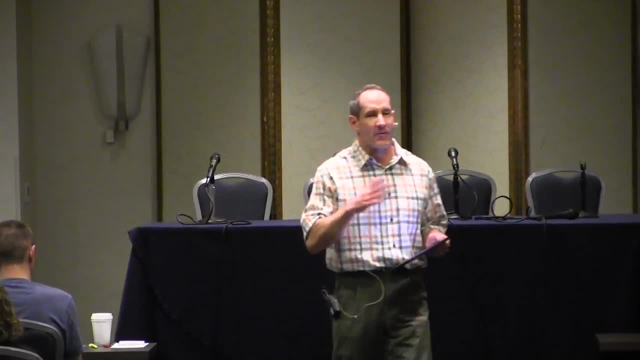 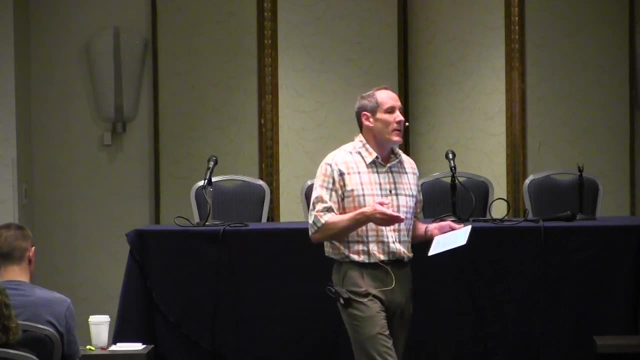 This is a retrospective, as Jerry would say. No methods. They just looked at charts on kids who came in And they got troponins on And, lo and behold, 17% had a positive troponin. Now that seems to me kind of crazy. 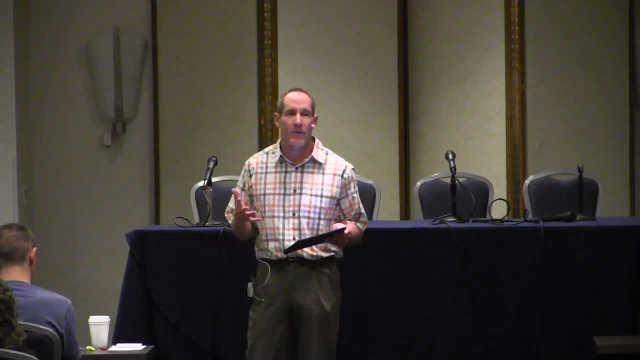 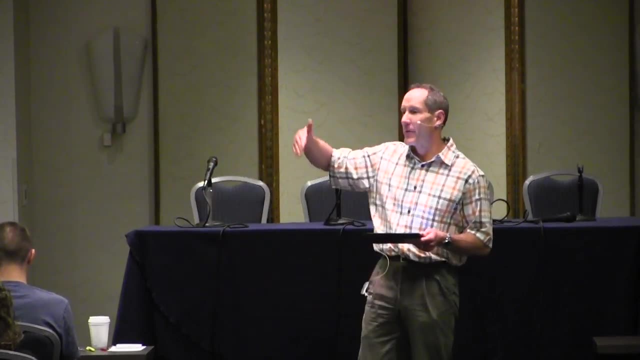 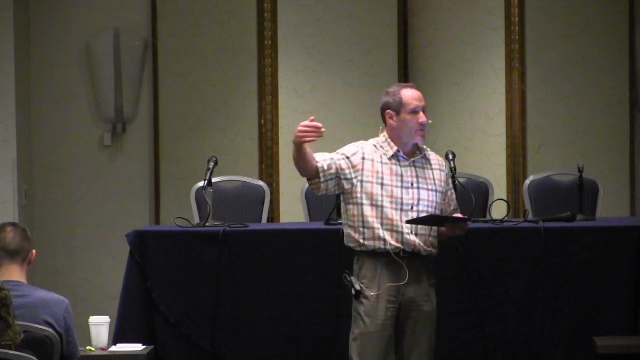 In a pediatric population to have 17% of them present with an elevated troponin. When they ultimately followed these kids, Less than half of the kids with an elevated troponin had a cardiac diagnosis at the end of the day. So that speaks to, I think, a few things. 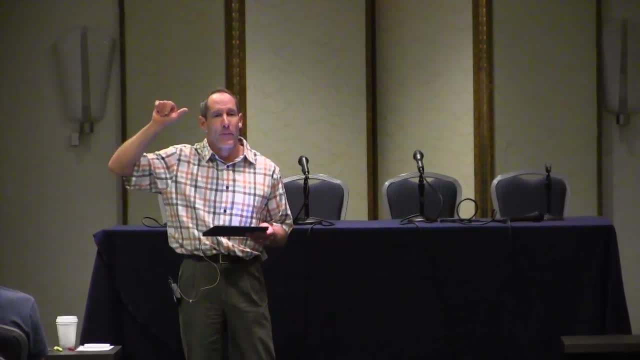 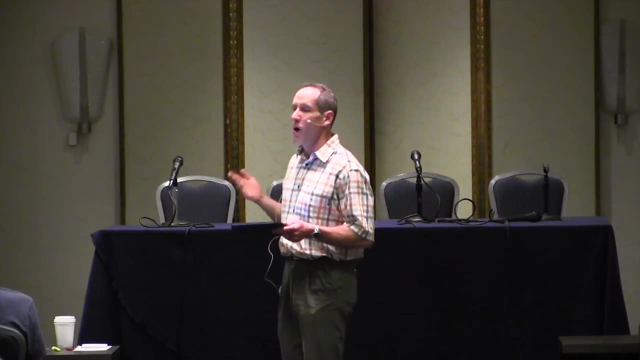 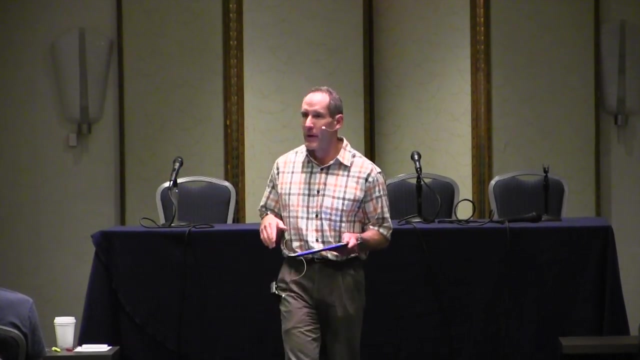 And we'll talk about this more in another talk- But cardiac troponins are becoming more and more sensitive, Less and less specific, And so when you have a patient population with a very low incidence of disease, A positive test in this case was just as likely to be a false positive than a true positive. 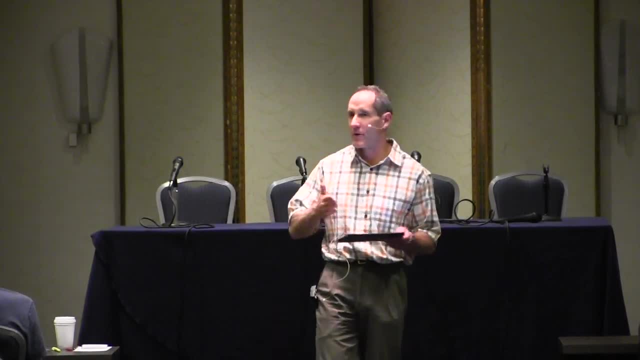 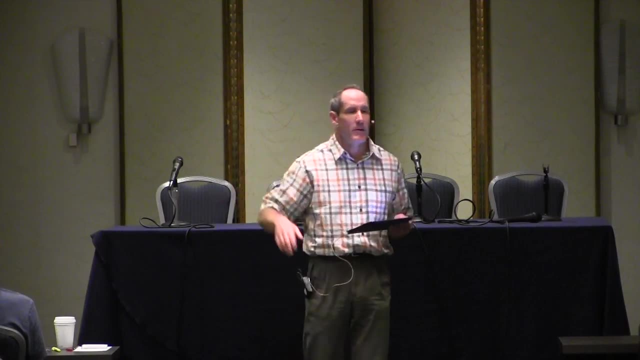 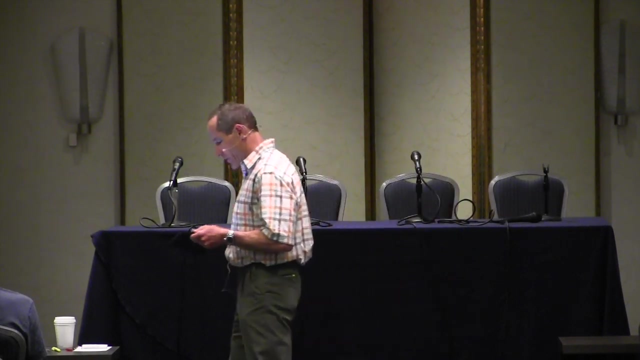 Troponins have a limited value in kids, In part because cardiac disease is so uncommon. And even if it's positive, It's only maybe half predictive of that being an actual, real finding. So, getting back more to the myocarditis, We have abstracts five and six talking about presentation of myocarditis. 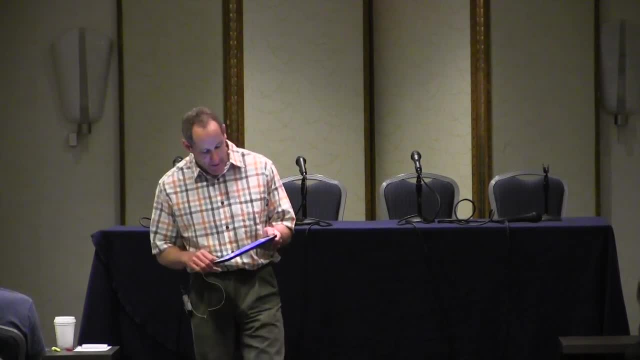 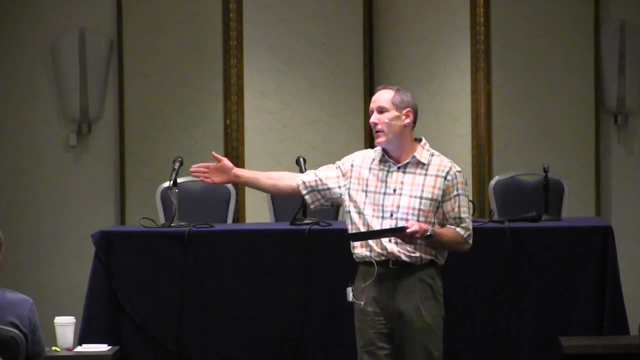 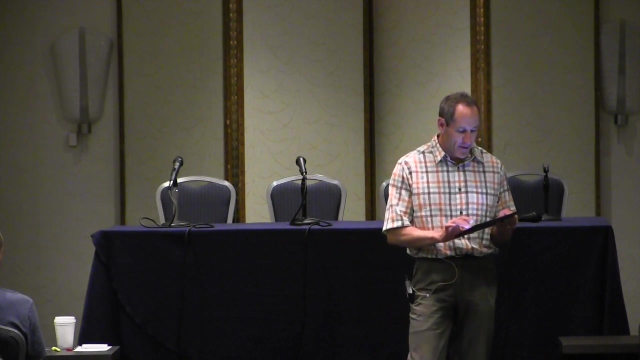 Two of these papers point out That about 50,, 75, 85% of these kids are not diagnosed on the first visit. So that gets back to my introduction. Rare finding of myocarditis. I think one of these studies was of a pediatric center. 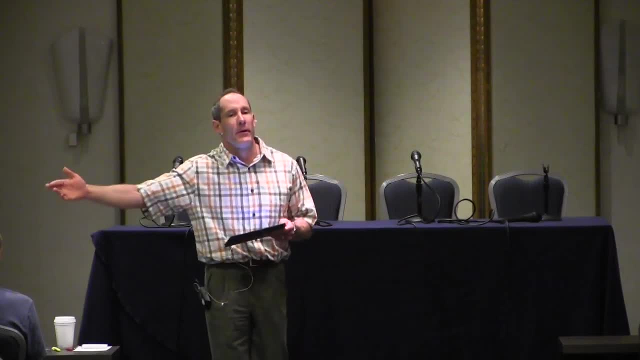 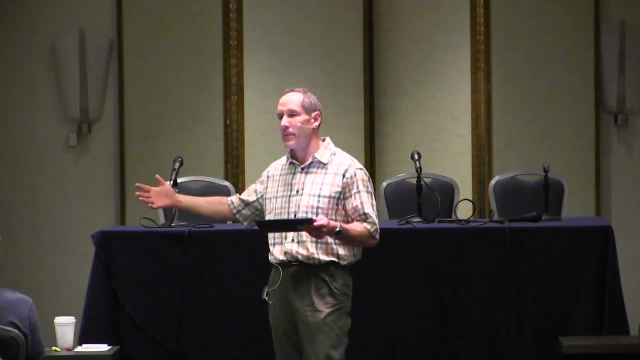 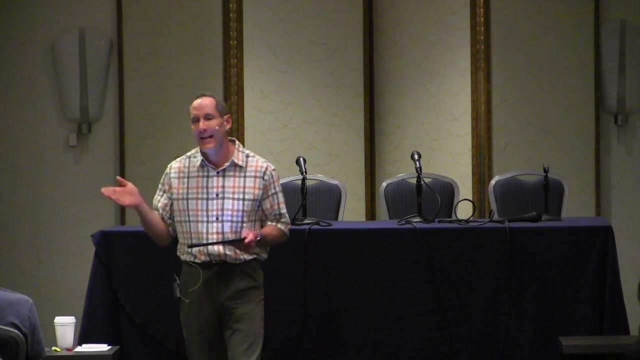 Actually a couple pediatric centers, Several years experience And they had 62 kids in this study. So you take a pure pediatric ED, You take a couple of them, You look at a few years And you can only find a few dozen of these types of presentations. 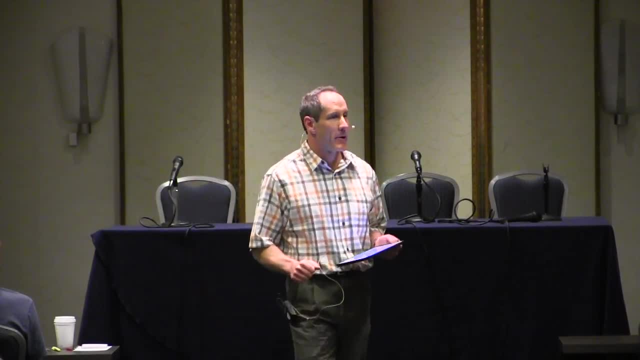 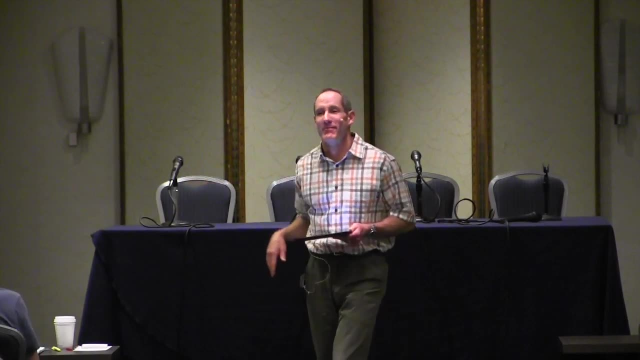 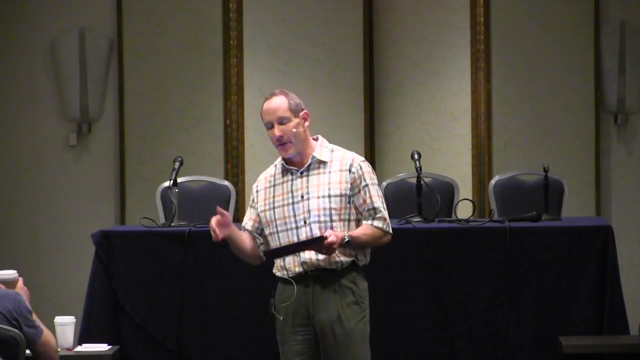 It's rare. Has anyone here ever actually seen pediatric myocarditis? We've got a couple, So cumulative experience of decades and decades, And you'll get maybe one in every five careers. So again, nothing we're likely to see, But something worth keeping in mind. 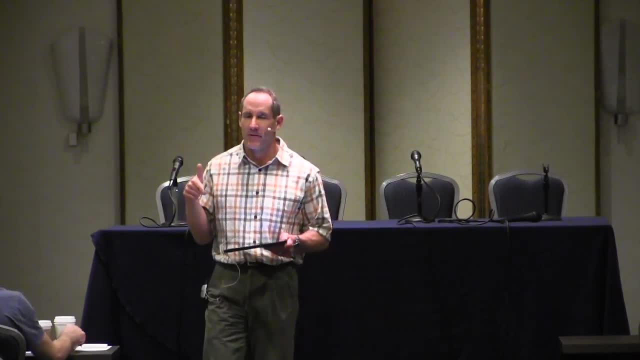 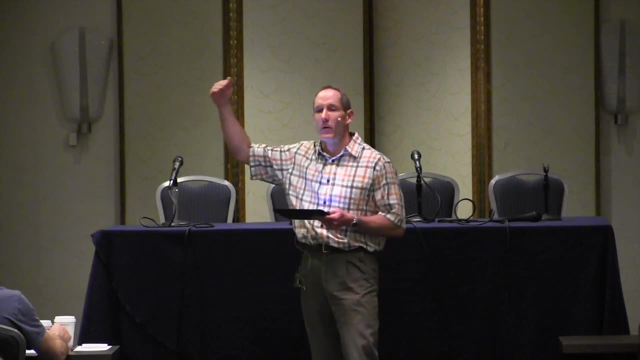 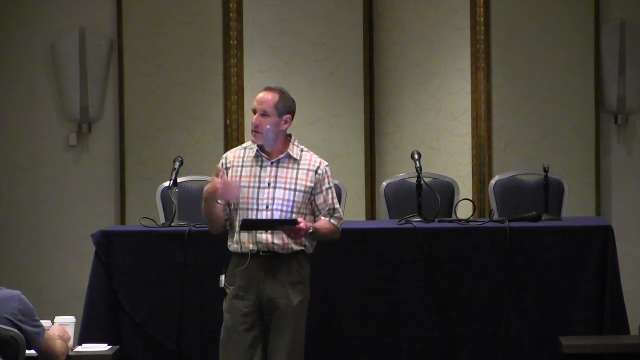 So The most common misdiagnosis in a couple of these studies Was pneumonia or some other respiratory complaint. So obviously the ratio of respiratory to myocarditis Is going to be almost infinite. But when you see a kid That just seems a little bit more dyspneic than appropriate. 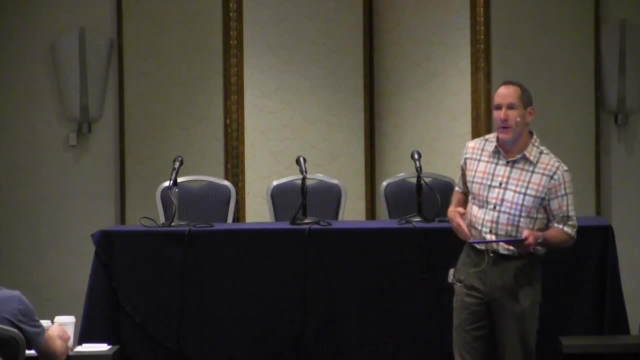 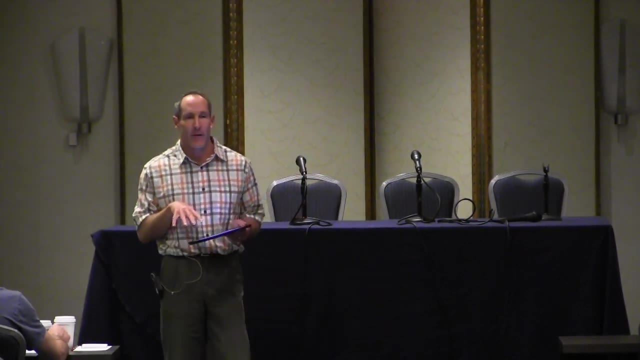 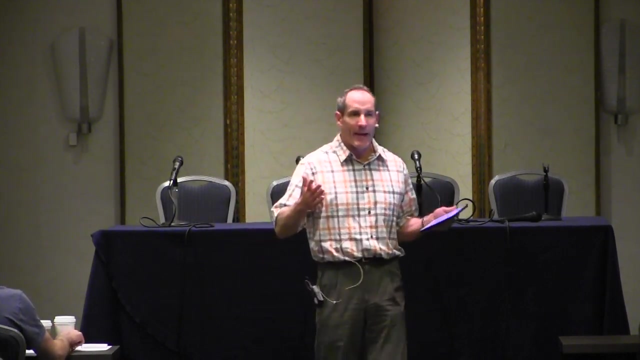 A little more tachypneic, Maybe feel for a liver, Because hepatomegaly is a fairly common finding In a lot of these presentations. I think one of these was something like 70% Had hepatomegaly And God knows how they found that. 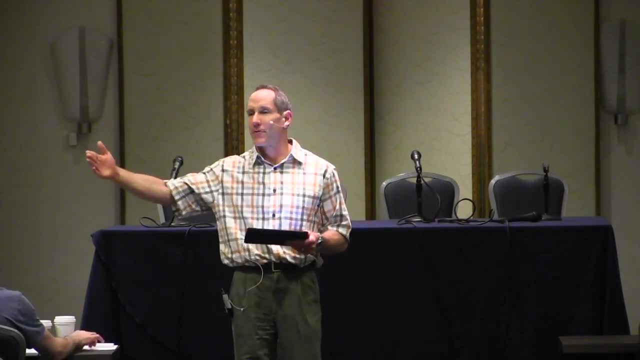 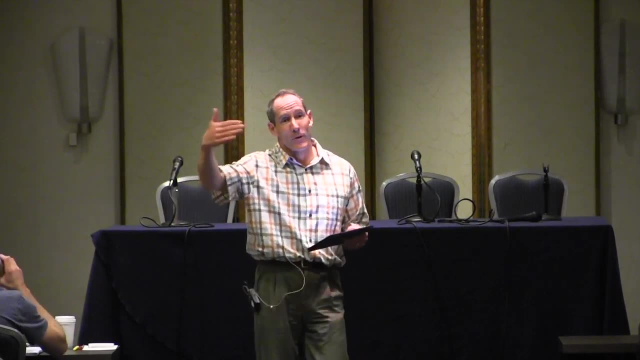 On probably retrospective chart review, And that was maybe after the diagnosis was made. Somebody goes back in and says: Oh yeah, Did you feel that liver? So the challenge And the real coup Would be To feel the liver up front. 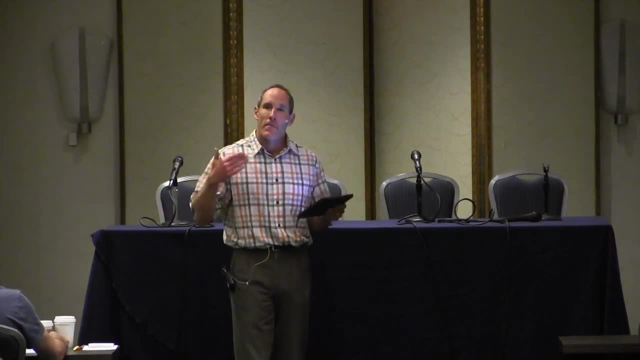 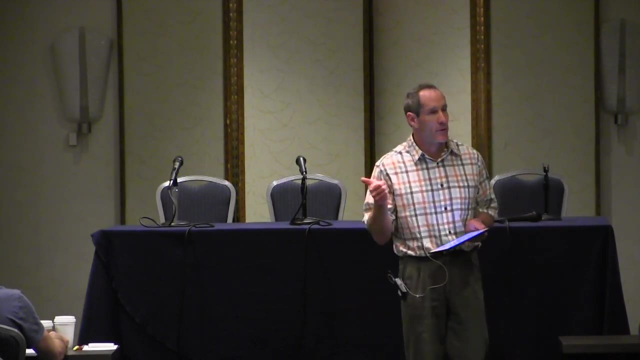 In the tachypneic kid And say, Gee, I wonder If this isn't just a viral thing. Chest x-rays: Chest x-rays are commonly abnormal. Cardiomegaly is the most common finding That you're going to see. 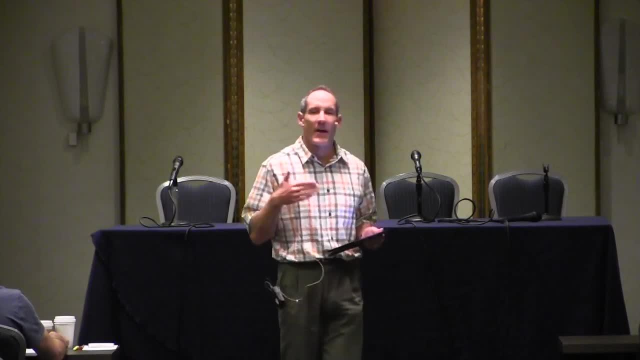 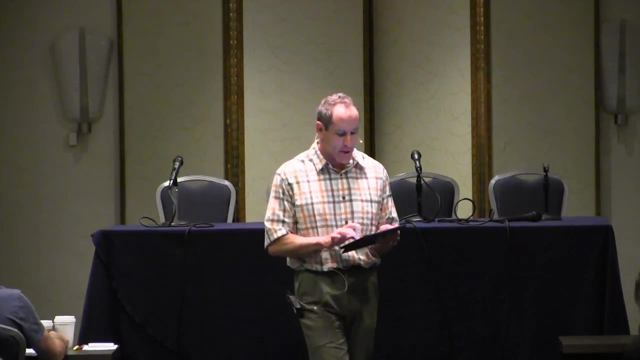 And EKGs are commonly abnormal, But in a very nonspecific way. So sinus tachycardia is what you're most likely going to see. One of these papers talks about axis deviation. I couldn't really quite understand that, But the typical workup. 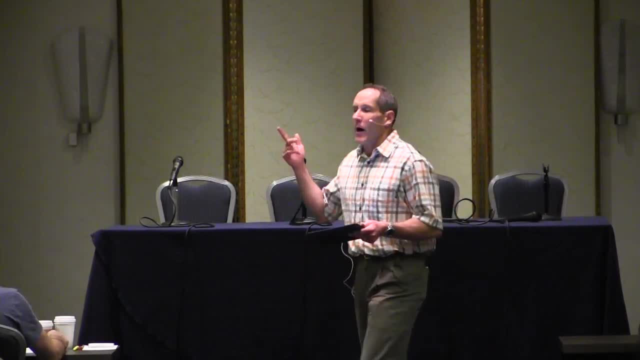 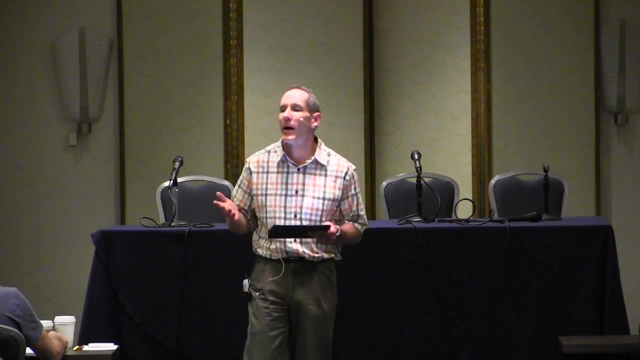 If you're worried about it Would be a chest x-ray. Of course, Everyone's going to get labs. AST, One of the liver function tests Was considered, Was found to be the most common abnormality. But something to keep in the back of your brain. 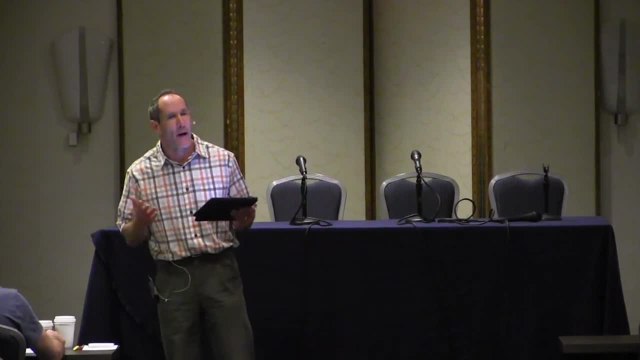 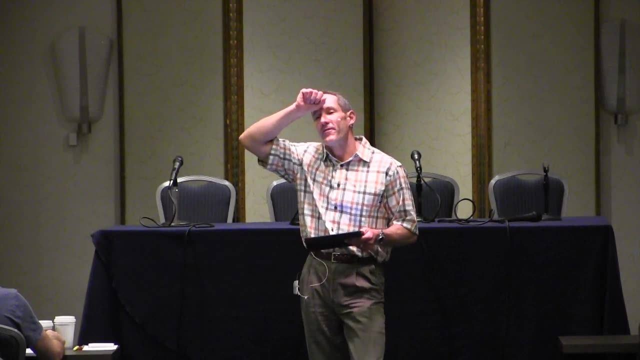 For the kid who comes in With shortness of breath And you're really not quite clear On exactly what's going on. One thing I did find disturbing, though. One of these studies said A third of the kids came in febrile. 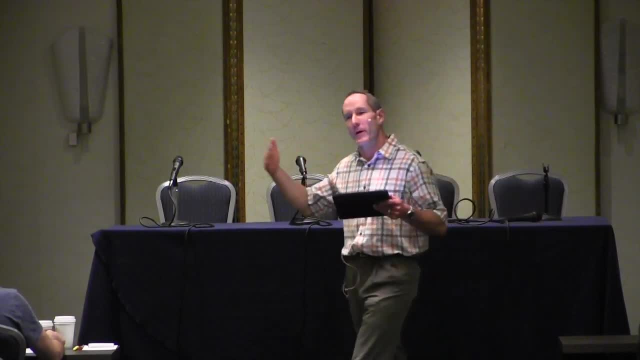 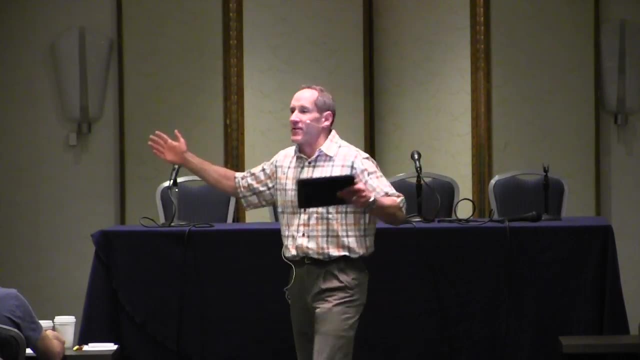 And I just didn't think that was fair, Because if I'm trying to distinguish Infectious from myocarditis And they're febrile, I'm just not going to get it. But beware that fever does not exclude myocarditis. And again, 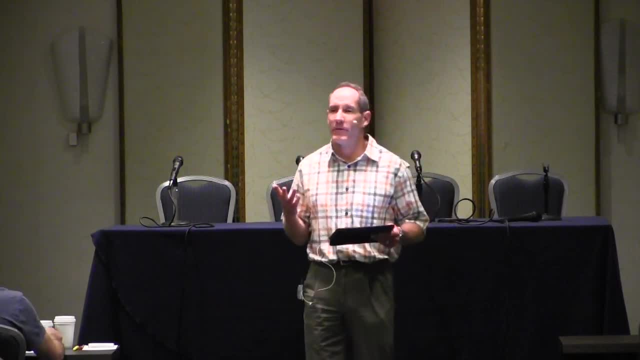 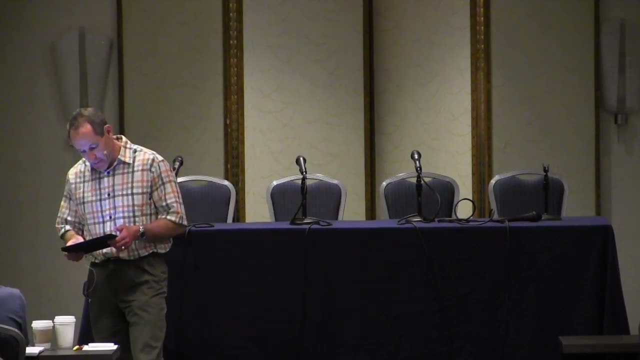 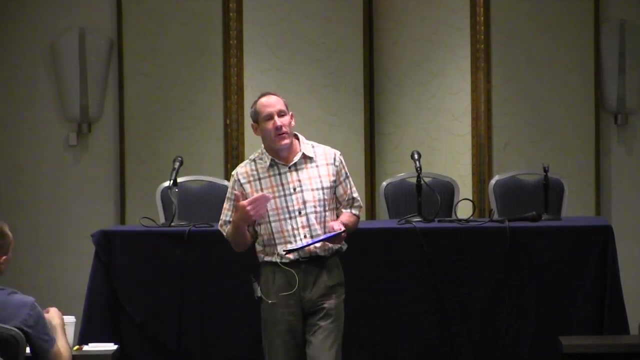 A third of the kids in one of these series had fever, Which again I didn't think was fair. Child abuse is the next topic. So those are abstracts. eight And beyond, And those abstracts don't necessarily Speak so much to our patient. 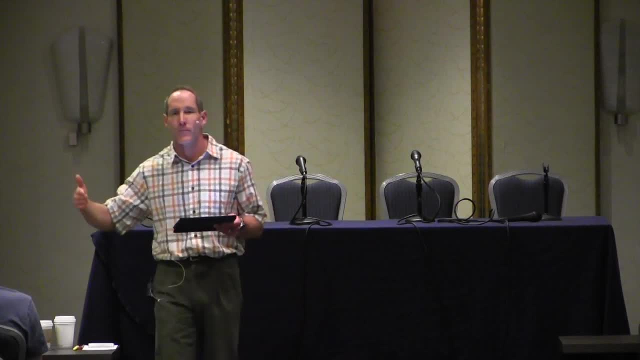 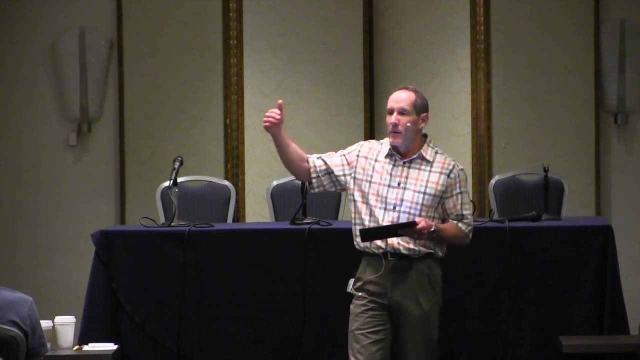 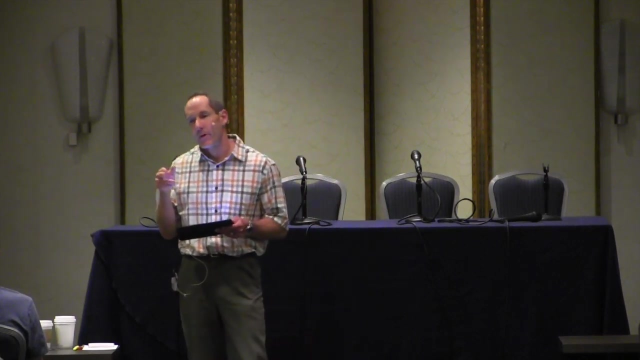 Physician, One on one interaction, But they talk more about demographics. I think it's important for us to realize that Pediatric abuse, Non accidental trauma, Is one of those things that matter, for a couple reasons. One is because, of course, the acute presentation. 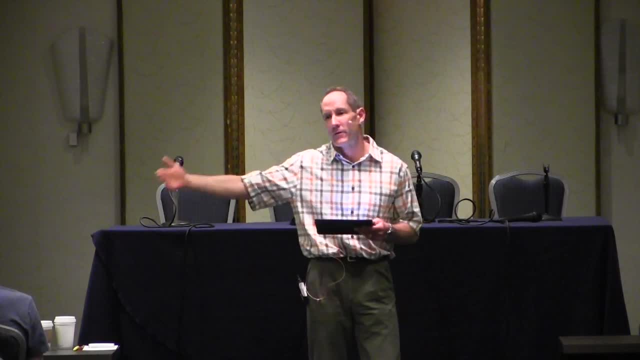 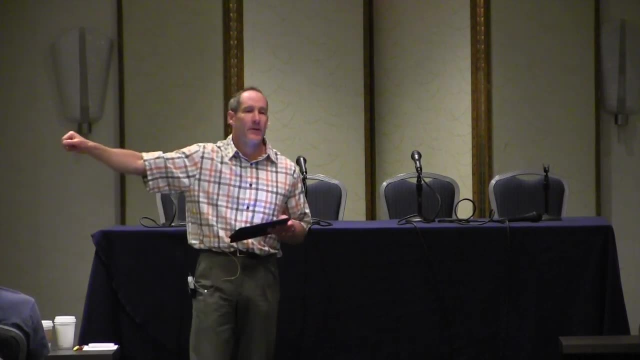 So the kids coming in And what's going on with the kid Here and today. But the other thing about abuse Is that If you miss the diagnosis And you return the kid to the environment of abuse, Then there's a fairly high risk. That they're going to come back, And they're going to come back more injured. A couple studies have looked at this. One found an 11%, One found a nearly 50% chance That the kids who are missed Come back. 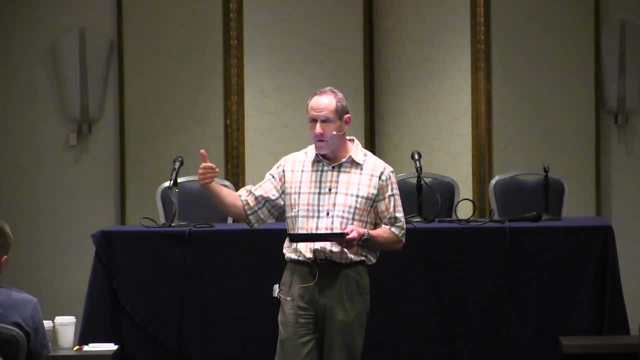 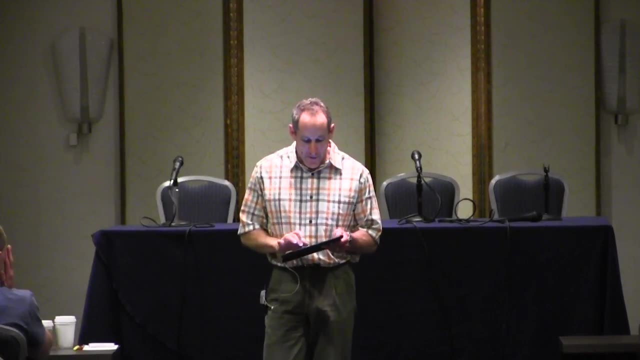 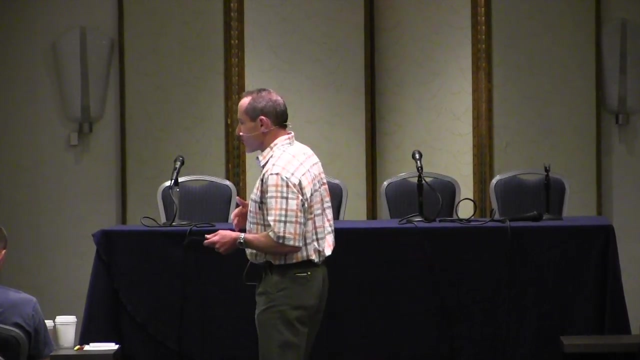 With more abuse, More injury. So it's very important for us to make the diagnosis Largely to prevent those downstream Consequences. The first three articles- Eight, Nine And ten- Are all by the same author And they look at screening in the emergency department. 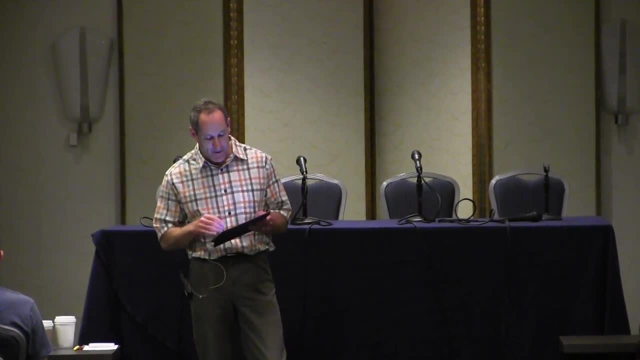 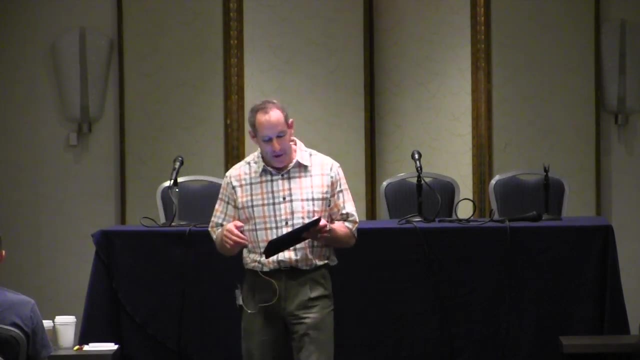 And it's a fairly wide database, So it's 39 or 40. Pediatric emergency departments Who do this all the time. Abstract eight was over 10,000 children Below the age of two Who were diagnosed with physical abuse. Another 10,000.. Younger than one Who had traumatic brain injuries And almost 3,000 kids Who presented with femoral fractures. So you had kids who they'd already made the diagnosis of abuse Femoral fractures, Which are considered a high risk injury. 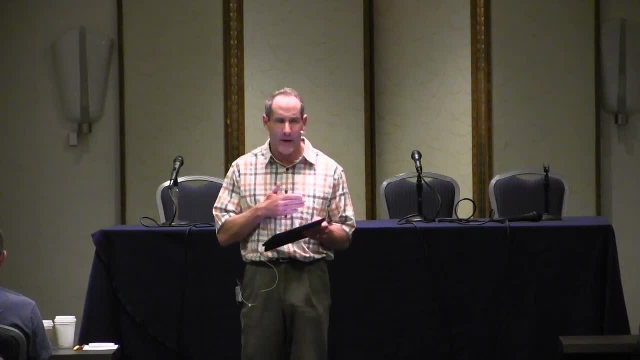 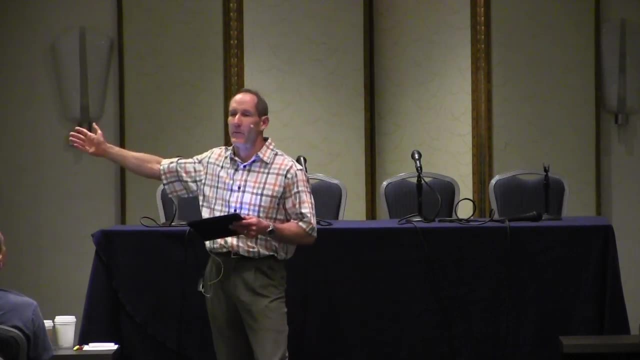 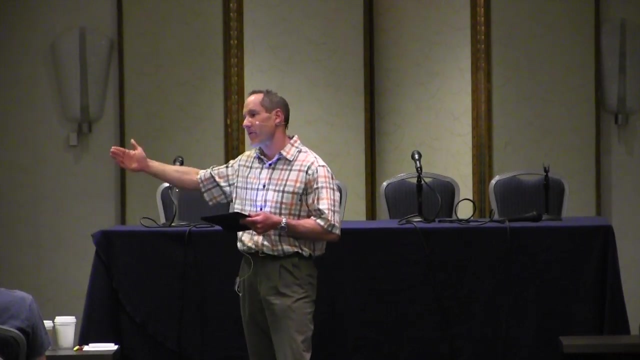 And then traumatic brain injury, And they looked at The individual hospital rates of screening And it was really very varied. So some hospitals screened almost everybody, Over 90% of the kids. Some screened only about Half And then obviously the fewer that you screen. 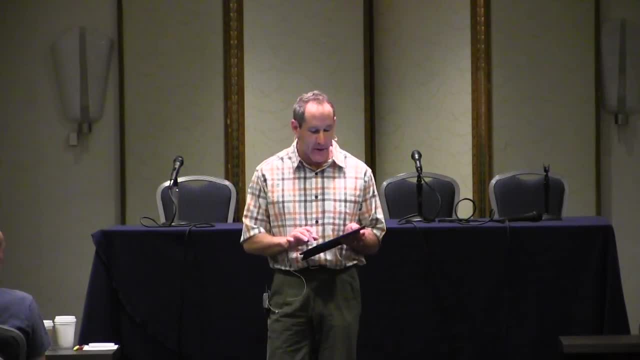 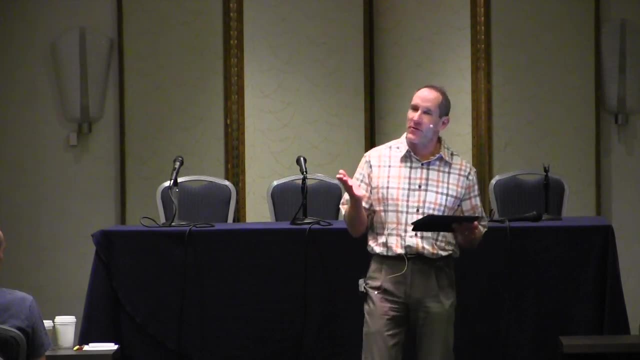 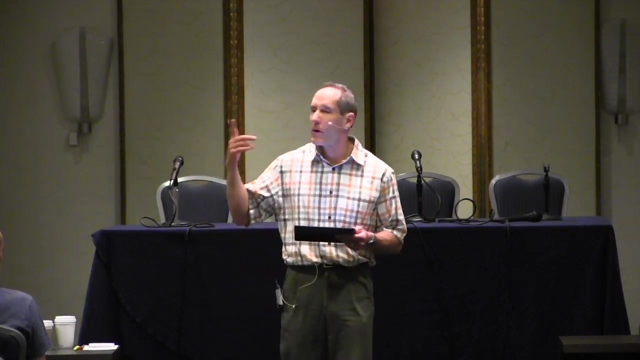 The fewer that you find And, what's more disturbing, As you dive into the data, As these authors did, There appears to be significant demographic Differences on who gets screened. So the poorer you are And the less white you are, The more you're apt. 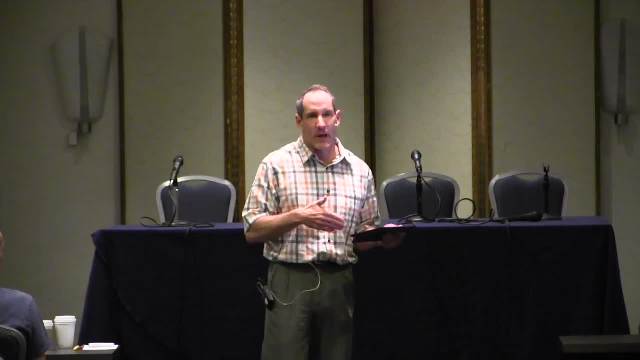 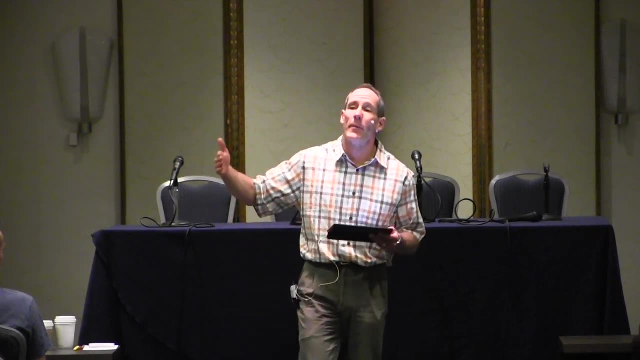 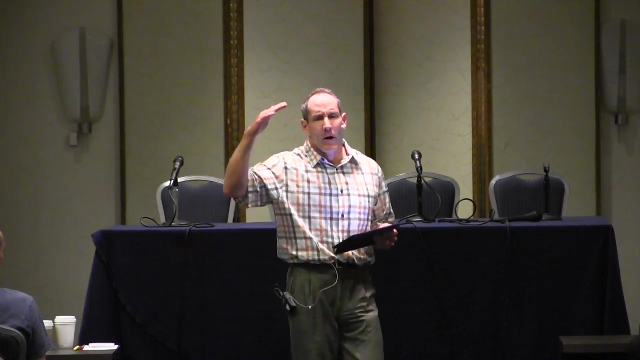 To get screened, And I think it certainly suggests- You can't prove it- That there are significant cultural biases For Who we think might be Subject to abuse. There was a great article in the New England Journal Within the last couple months. 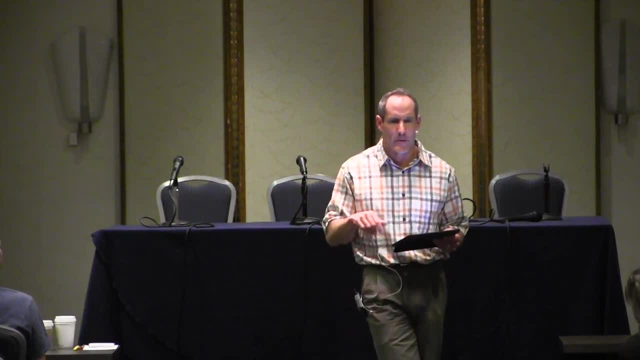 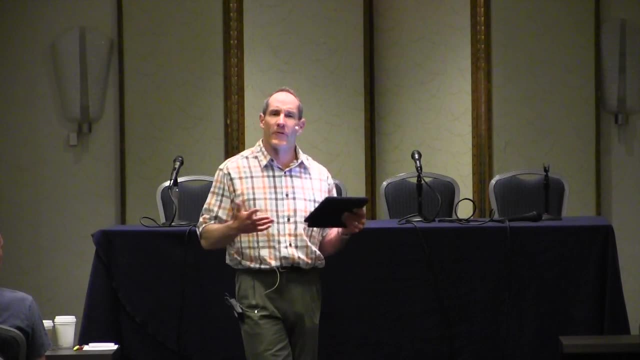 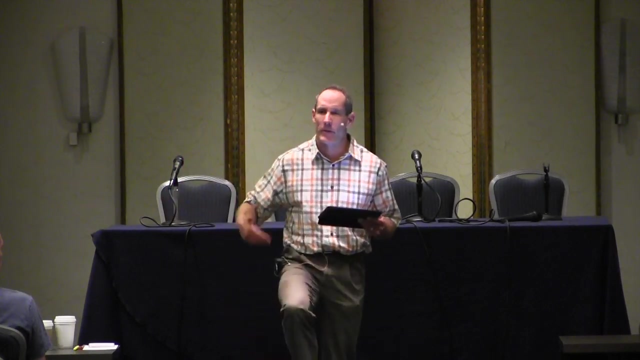 Of a female Emergency physician Who Wrote up this Very moving story Of seeing this kid from an upper white Background. And there was everything there And traumatic brain injury And multiple rib fractures And the Hemorrhages in the retina. 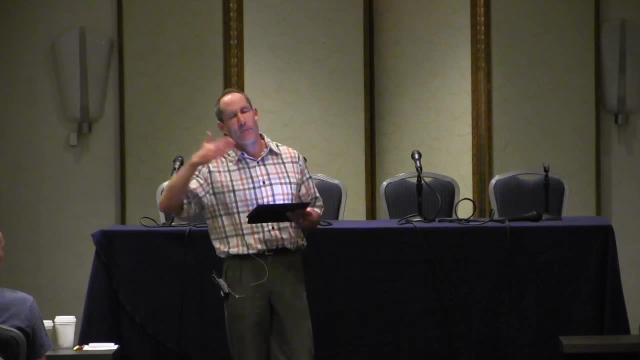 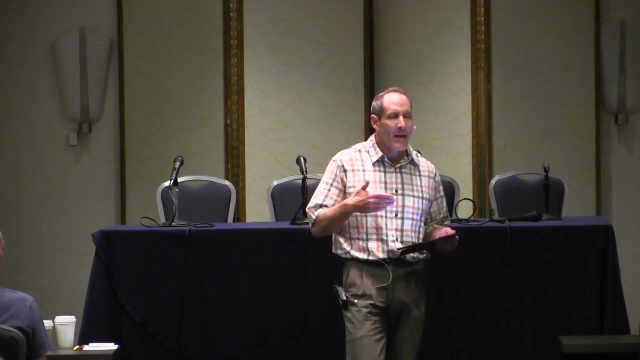 And it was her struggle To come to grips With the notion that This beautiful looking family Could do this to the kid, And I think one of the things That's good for us Is we don't have to come to that conclusion. 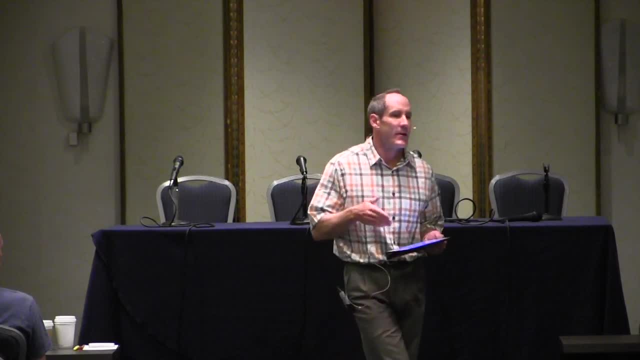 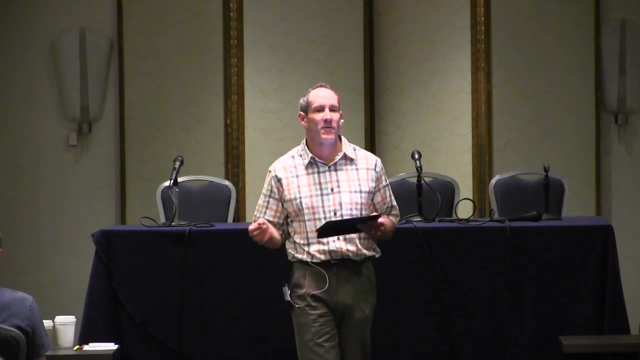 So one of the points Of one of these articles Is that it's rarely necessary For us To make the diagnosis of abuse, Or for the diagnosis to be made Within the first few hours. Our job is to trigger the process. 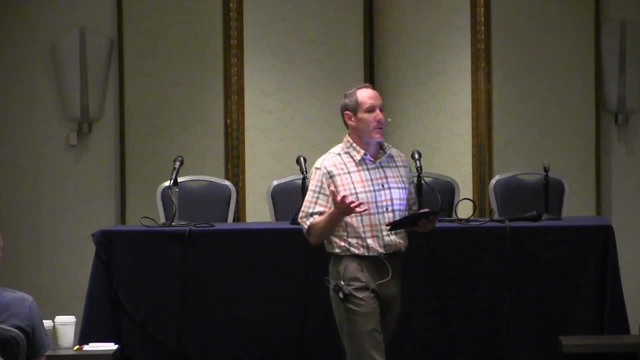 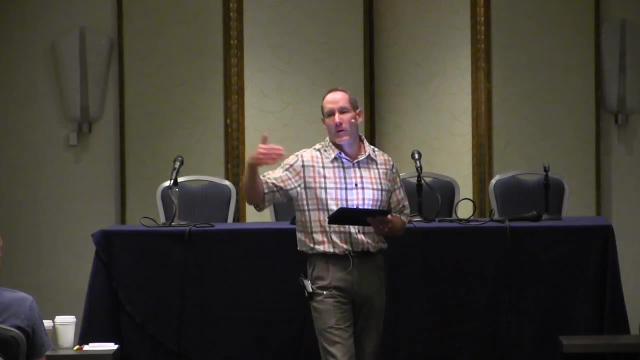 Involve child protective services In a non-judgmental manner. I think it makes it much easier for us to say: You know, Whenever we see this, This is what we do, So you don't have to be the accuser. 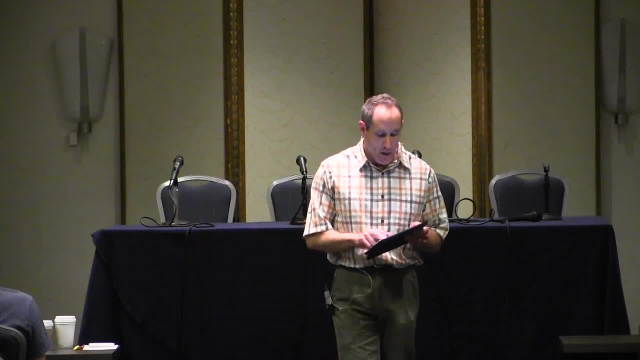 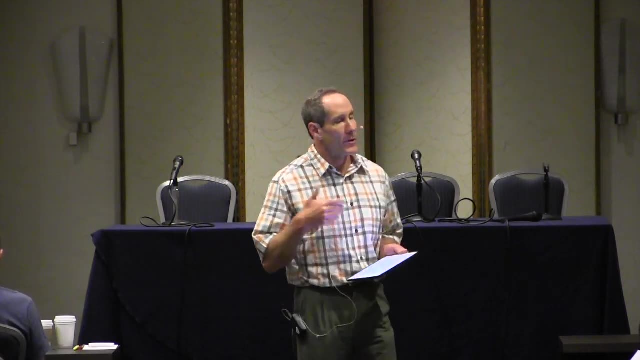 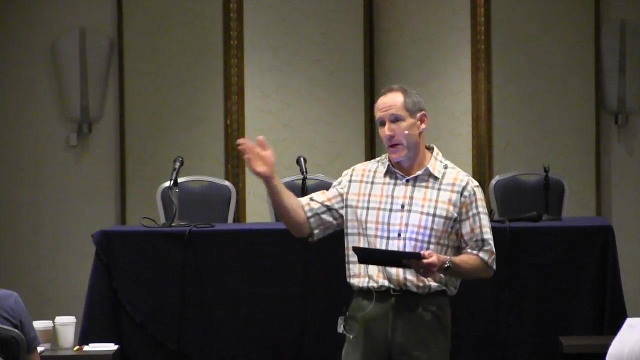 You just have to recognize the potential And trigger the process. One of these articles Is about the lags Of child abuse. What are some of the things you all look for When you're considering it? Inconsistent stories, So story changing over time. 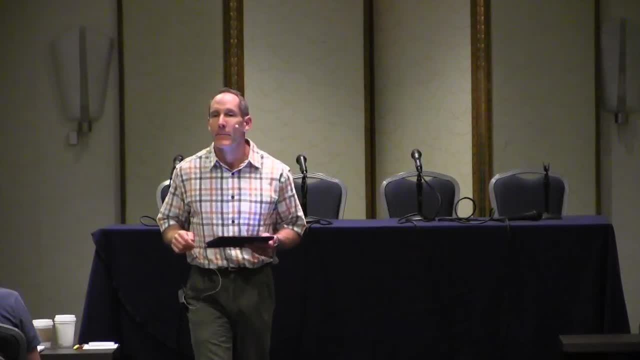 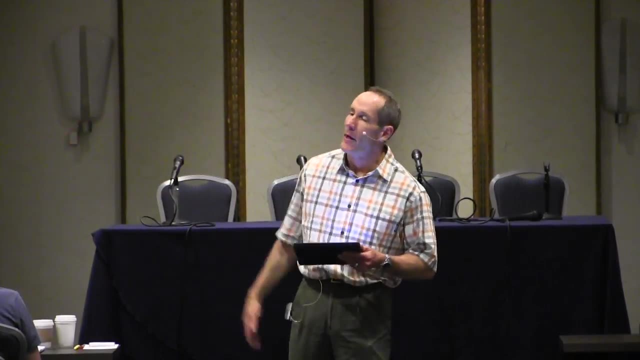 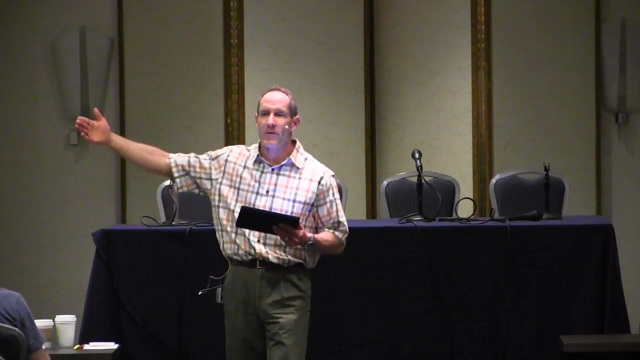 Different people telling different things, What else? Delayed presentation. So this talks, I don't know Somewhat randomly about a presentation 72 hours or beyond As a red flag. Multiple visits, So previous injuries: Gee, we saw Bobby in here two weeks ago for this. 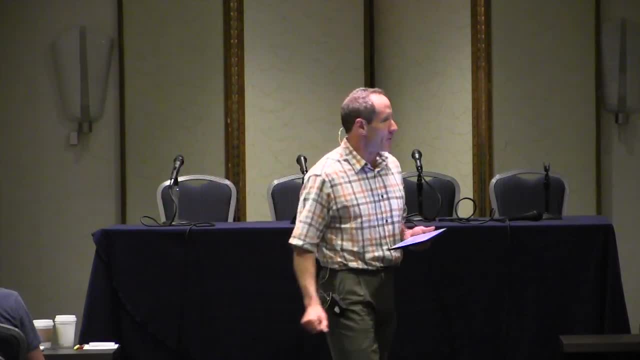 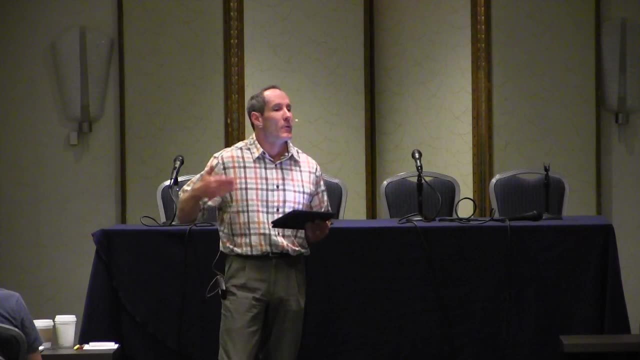 And then another one. similarly Would be previous involvement With child protective services. So those are some of the red flags And, like a lot of stuff we do in emergency medicine, Red flags for back pain. There are certain triggers That again non-judgmentally. 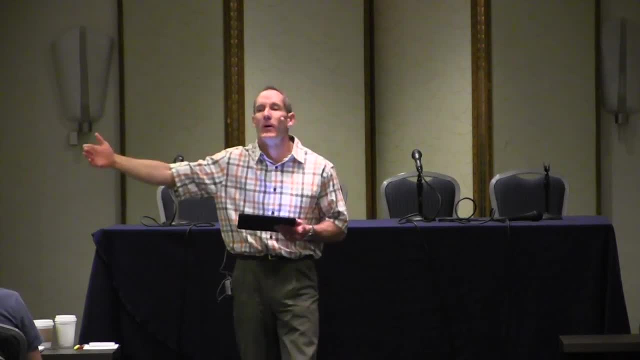 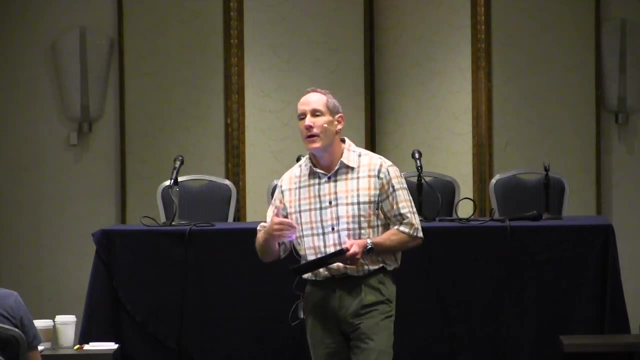 You can just say, look, When we see this, This is what we do. This is the best thing, The best way to approach child abuse And to try to not walk in And do that kind of global. Oh, what a happy, nice family. 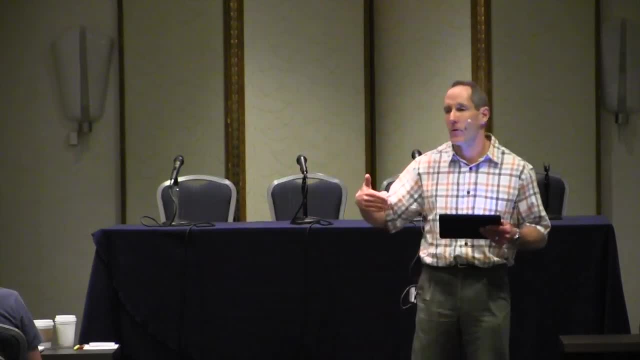 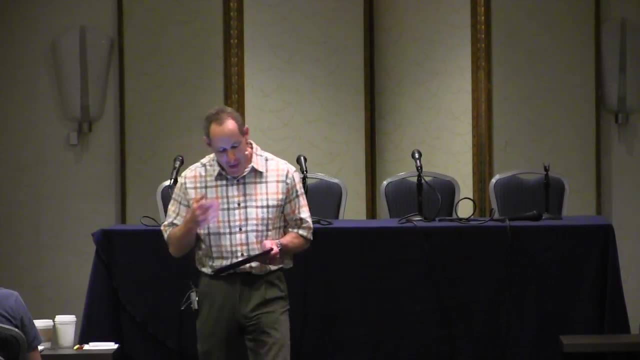 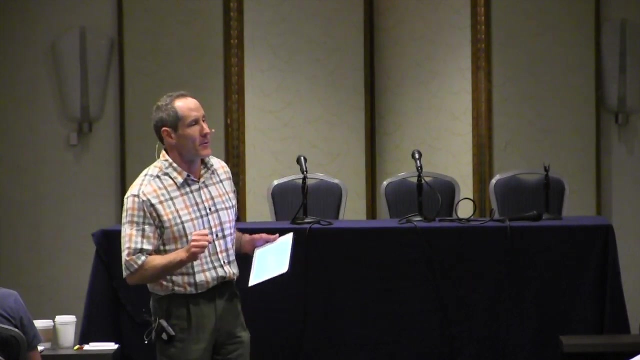 We've got here And just be your Usual clinical, Impartial self. There are a couple articles, A couple articles here Looking at bruising in children, And I think this can get to the CSI Kind of person in you. 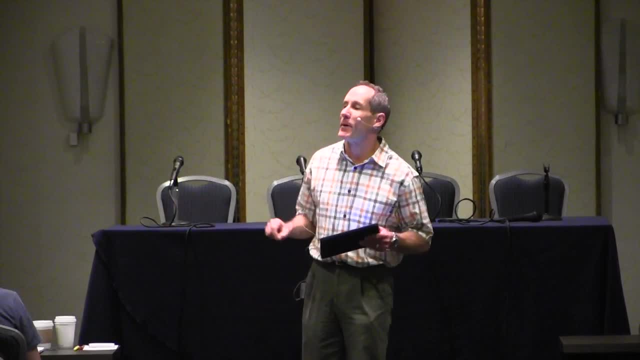 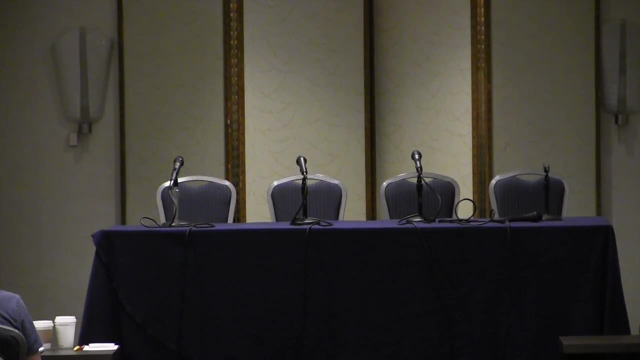 If you like to say: You know, I think I can tell by this bruise Exactly the mechanism of injury, Which would be really cool, But I don't think we can actually do that. So apparently There was some kind of teaching. 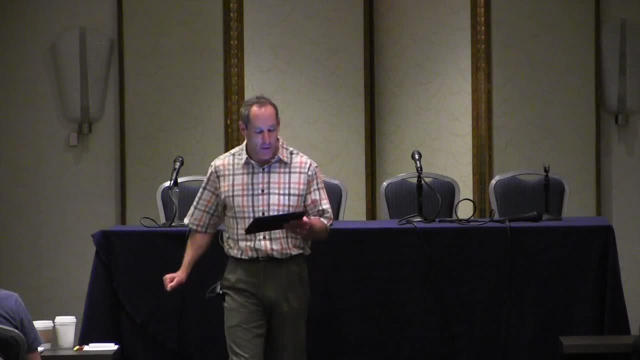 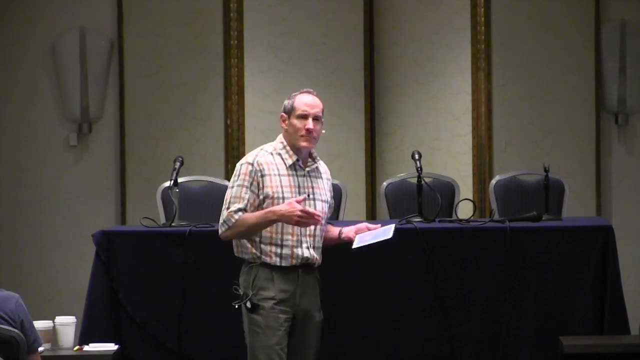 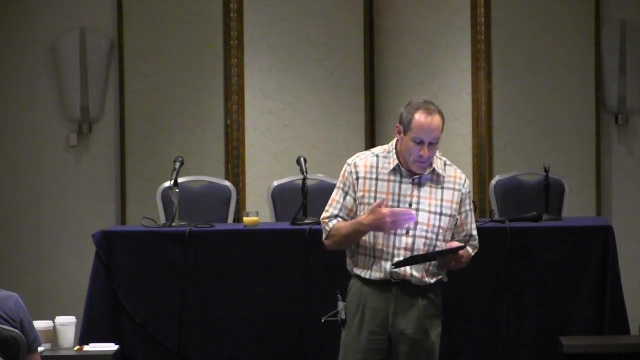 Which I was never taught, happily, Because it proves to be wrong That if you don't see bruising You don't have to worry so much about abuse. Had anyone ever heard that? I guess it's some kind of maxim. Maybe some people have taught. 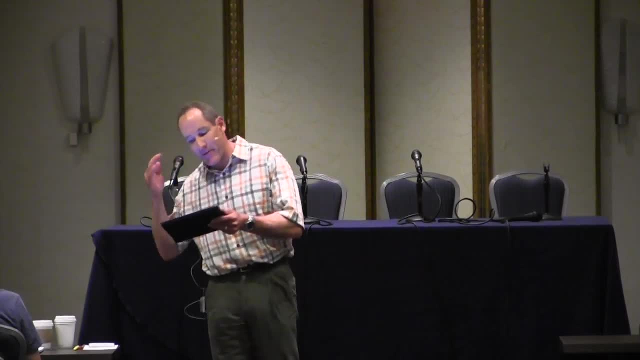 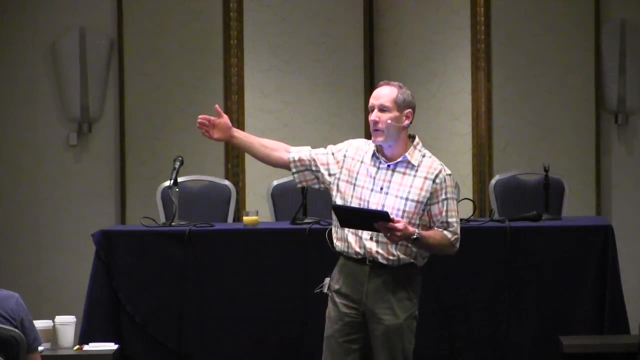 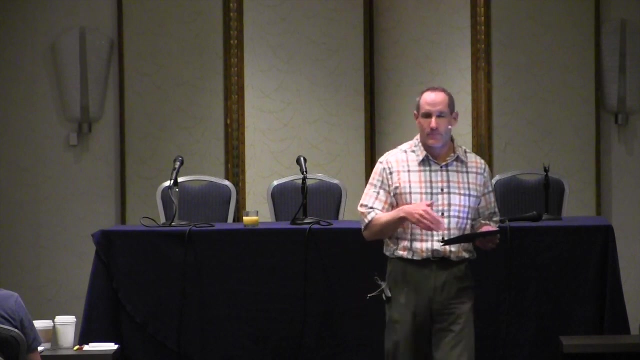 But abstract. number 11. Clearly talks about the absence of bruising Does not mean The absence of abuse. So they looked at kids And ultimately, however, they adjudicated That kids were abused or not. They tried to examine The pattern of abusing. 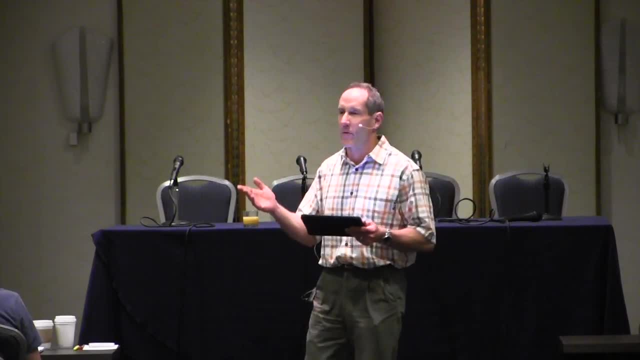 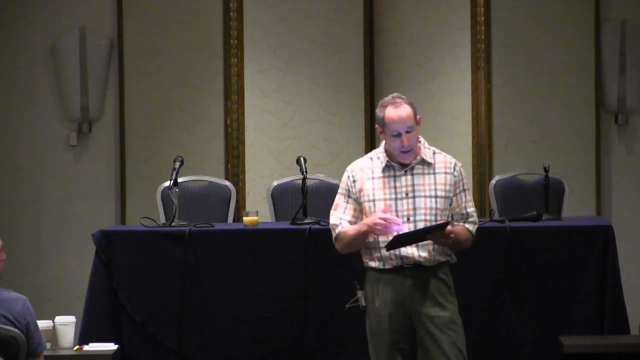 And whether there was bruising. Whether there was not bruising Associated with fractures Really didn't seem to influence the ultimate diagnosis That much. So I read an article. I thought it was a little bit more interesting. And there's a little table in your handouts. 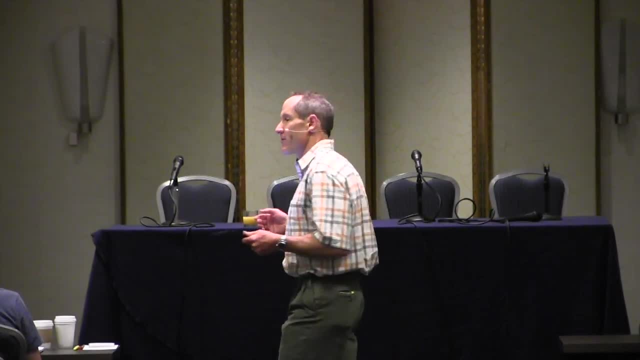 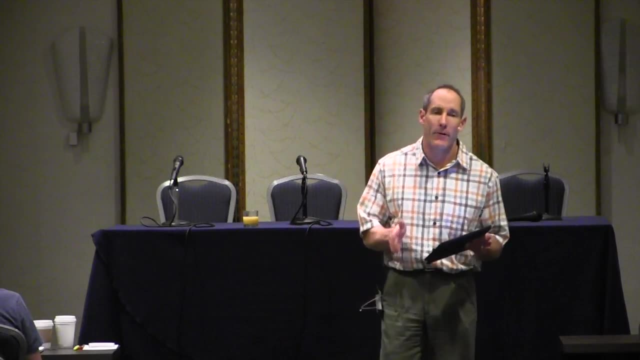 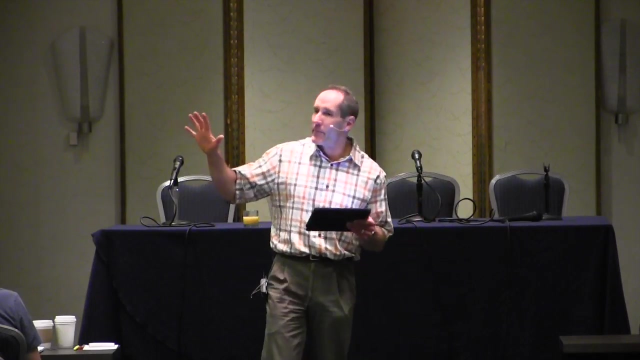 So it talks about certain patterns Are more highly associated with Physical abuse And I think if you see, As they point out, Distinct pattern of bruising, So obviously if you see a hand print On the kid's thigh Then that's probably a hand that made the bruise. 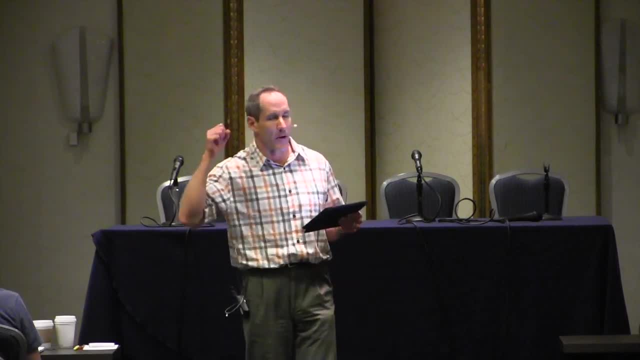 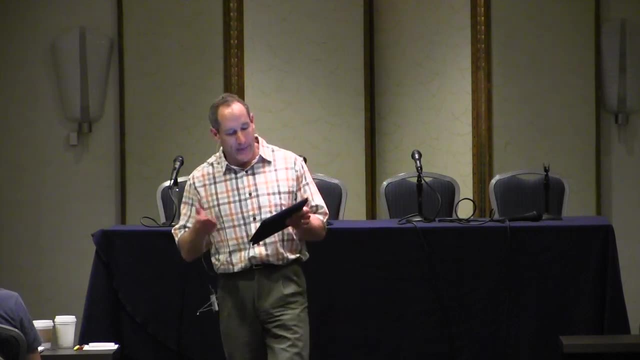 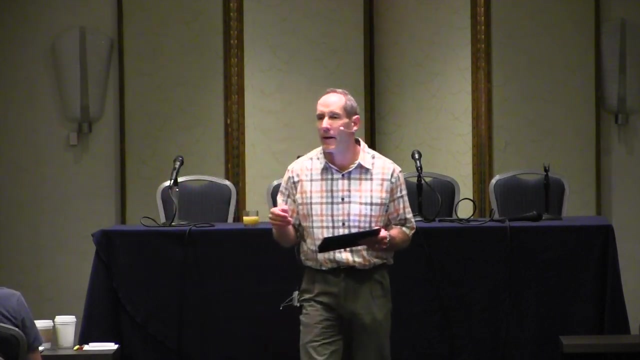 And similarly If you see other patterns- Hair brushes and that sort of thing- Something to think about. They found petechiae Were about eight times more likely In abused patients Than not. Of course, some of this might be incorporation bias. 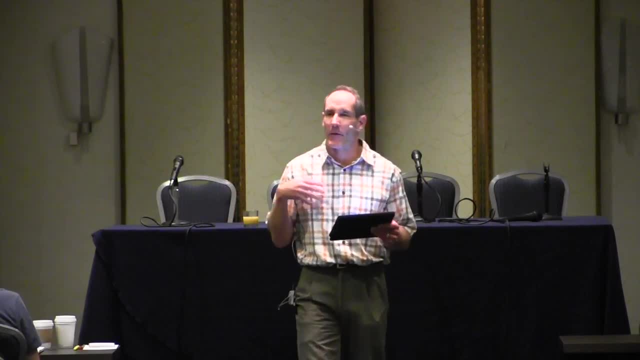 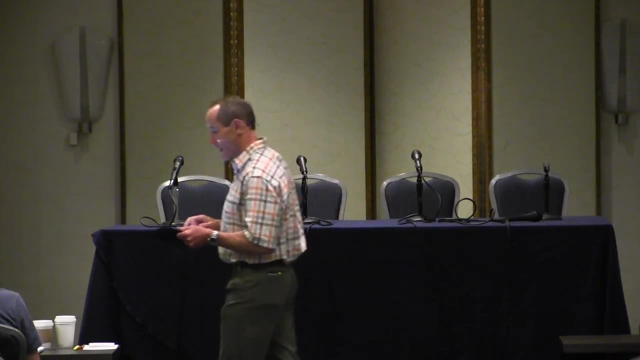 That when they saw these things, They already had it in their mind That that was probably more abuse. But in any case, Something to just put in your quiver If you want to pull it out at some point. Some things I thought. 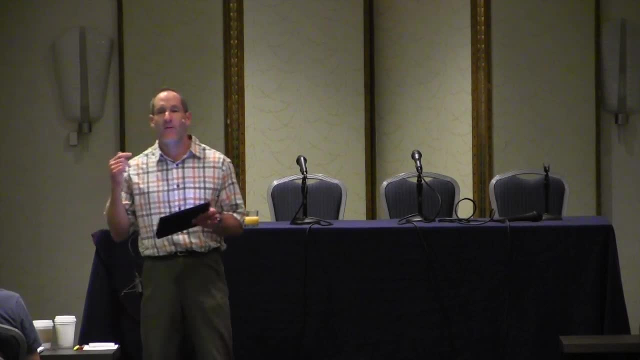 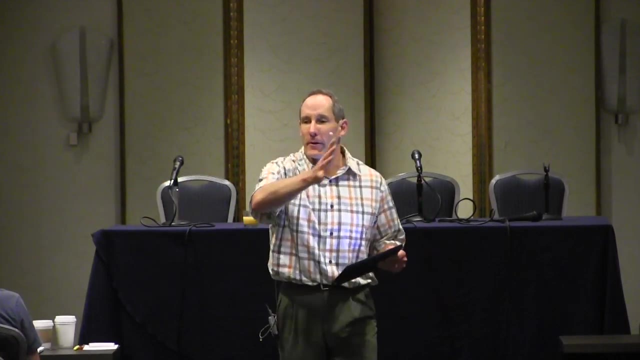 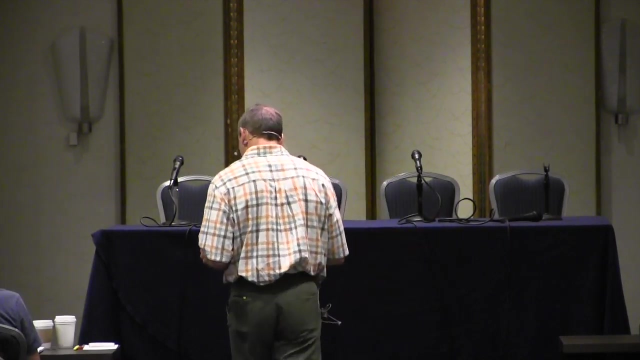 Were interesting was that Left ear and face Bruising was more common. And why would that be? Yeah, If the parent is right handed Or the caregiver is right handed, That will end up with less sighted, Trauma And then injury to the genitalia. 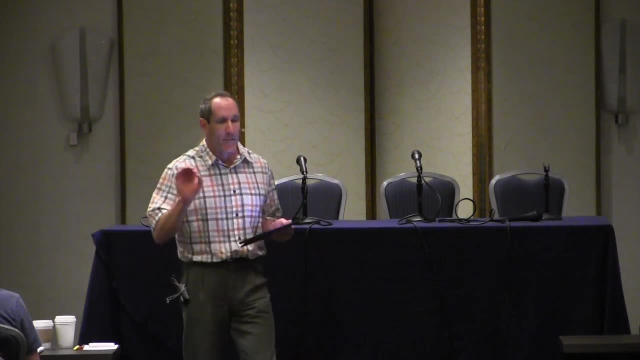 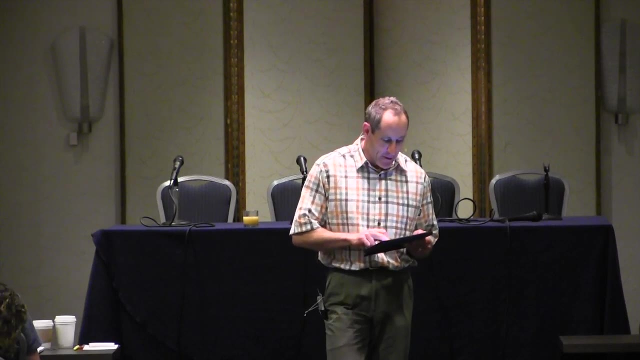 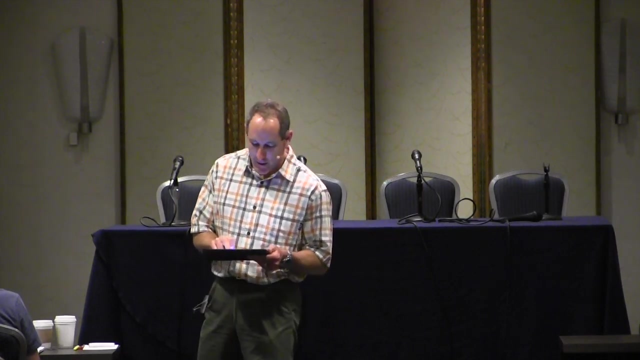 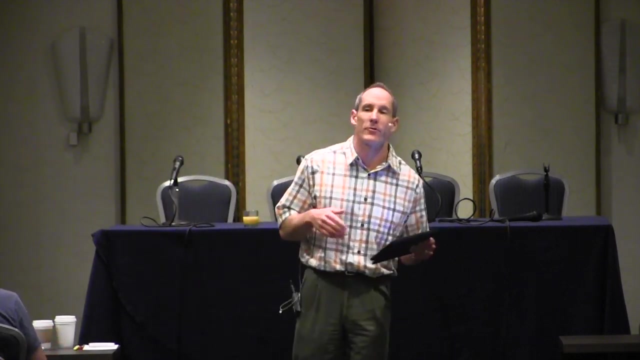 Or buttocks Less commonly Accidental. There is one paper here I'll just mention To debunk Article 13.. Should ask, Supposedly ask the question: Should we screen automatically For blunt abdominal trauma, Intra-abdominal injuries? 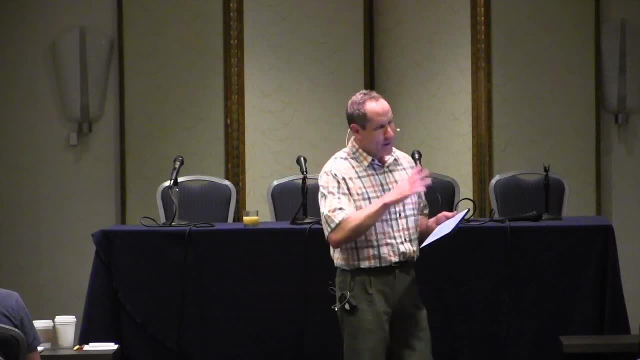 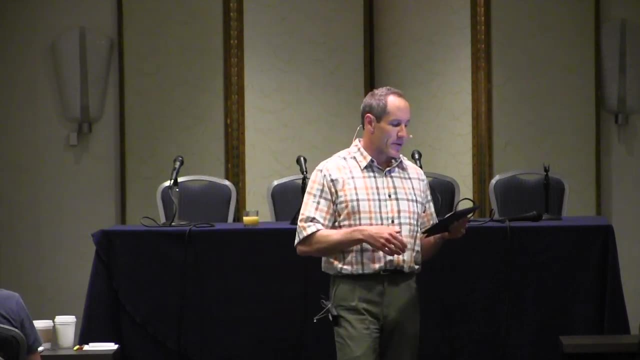 In patients in whom we are suspicious That might have been abused, And they do all kinds of weird Chart review stuff And they said, yeah, We think it should be done, Though ultimately, in their series of 244 kids, They didn't find one. 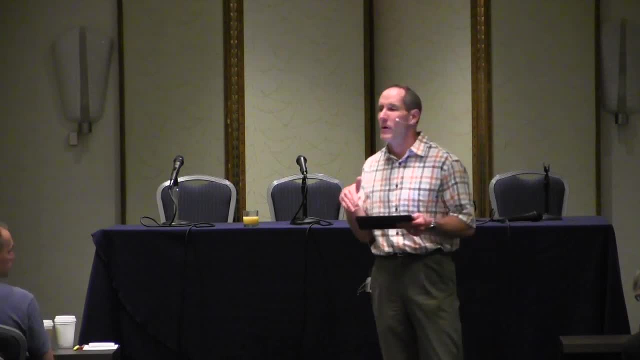 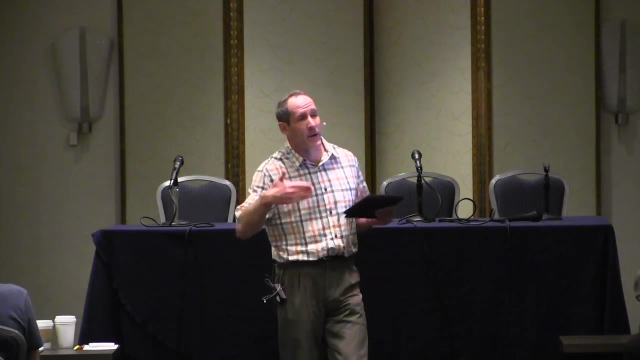 Because of their abdominal injury. So I think The only thing this article tells you Is that, despite what the authors tell you, They didn't have any And so they can't really tell you There's any good reason to screen. I think my take away would be: 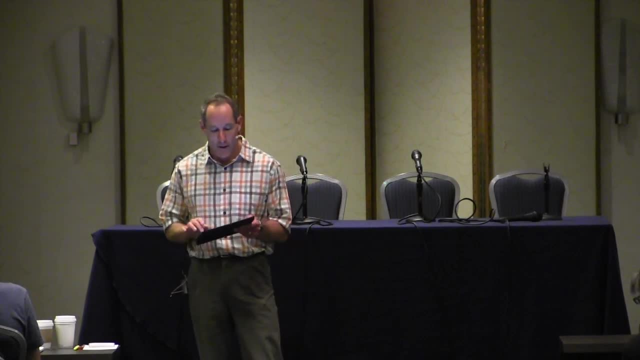 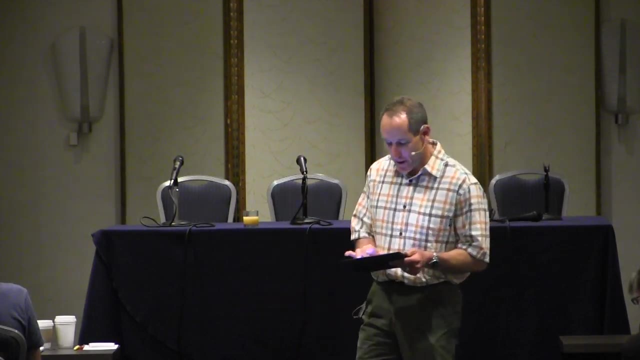 You do your clinical assessment on kids And then you go from there And of course, we now all have ultrasound, So that's an easy thing to add in. I'm going to end with Probably also not one of my favorite topics: The errors of metabolism. 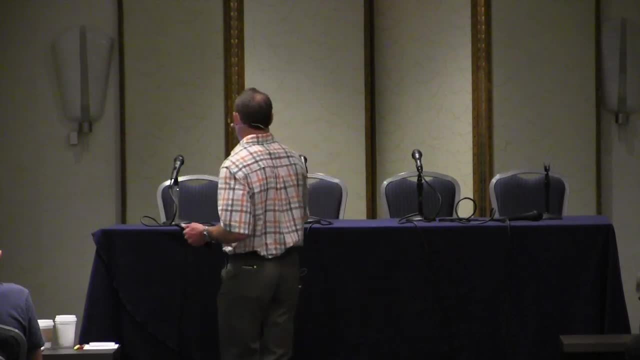 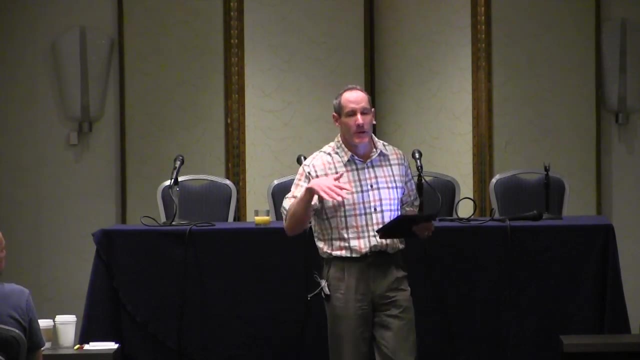 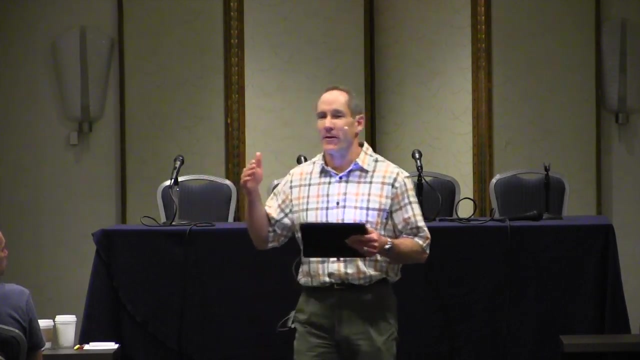 And I'm reminded When I, I think, the last time I was recertifying In emergency medicine, One of my study techniques Was: I went on to EMRAP And I just continuously Listened to EMRAP For months. 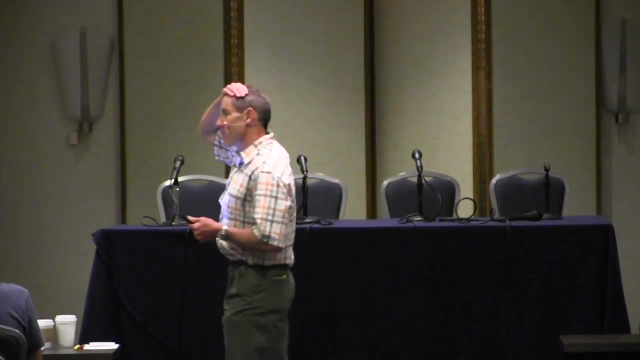 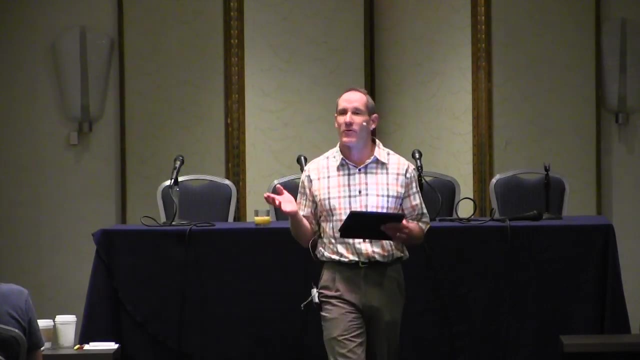 And it drove me crazy after a while. But at one point I got into this lecture Of inborn errors of metabolism And whoever was giving the lecture Was just going into it And I never understood it anyway. And then, as I'm, 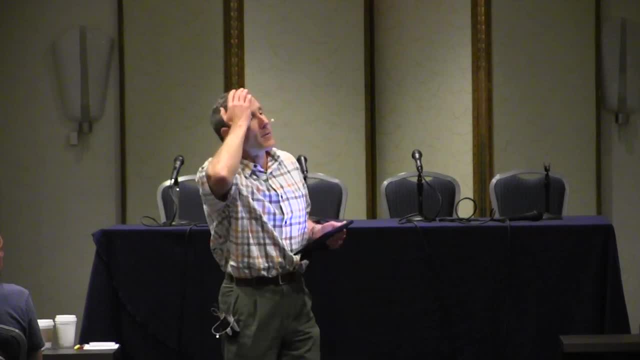 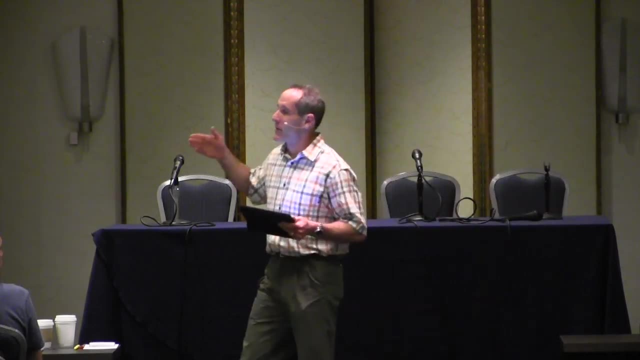 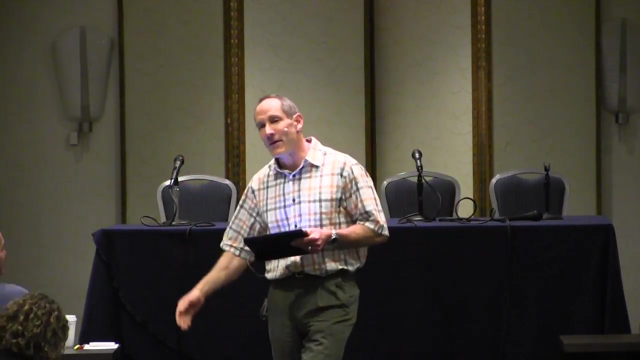 I think I was walking my dogs at the time And as I'm walking along Listening to this lecture, I said to myself: Oh my god, You are killing me. And at that moment Mel Herbert broke into the lecture And he said: 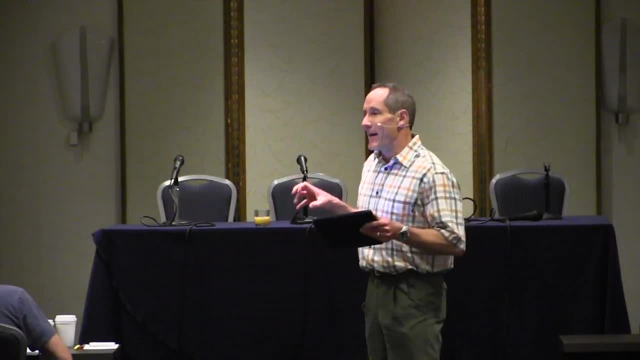 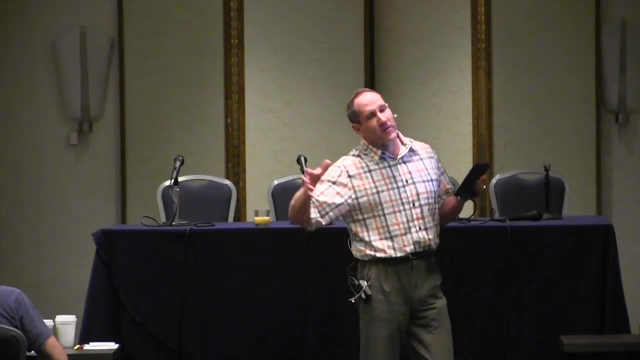 You're killing me About his own lecturer. So I think what I learned from that lecture Is that you can drown in If you really get into it, But you can also step back And take a global picture Of what is. 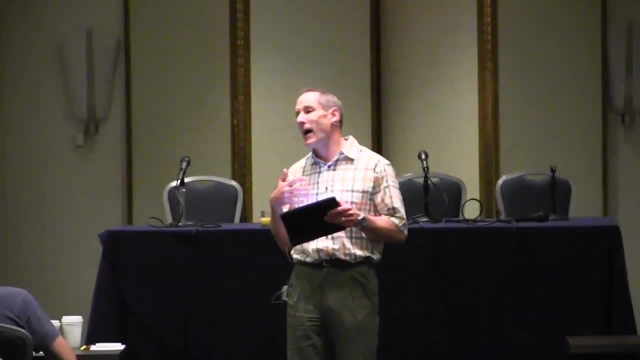 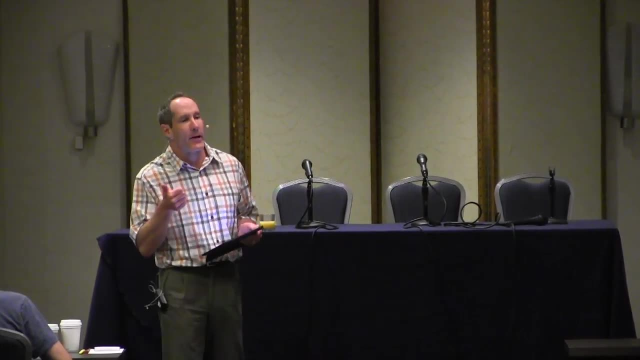 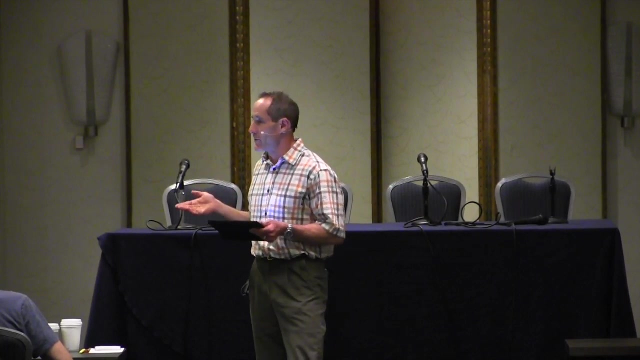 An inborn error of metabolism In general, And how, in general, does it present? And Toward that end, First of all recognize that it's fairly common, Which surprised me: Supposedly one in about 4000 births Will have an inborn error of metabolism. 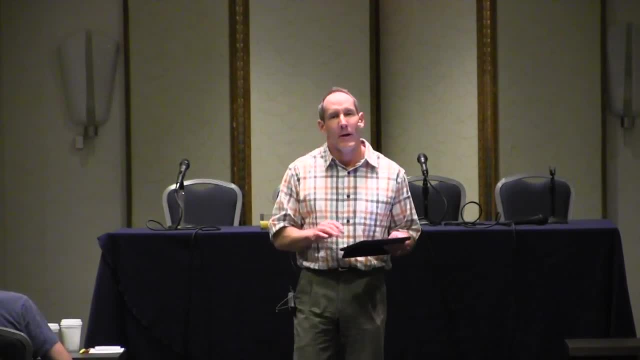 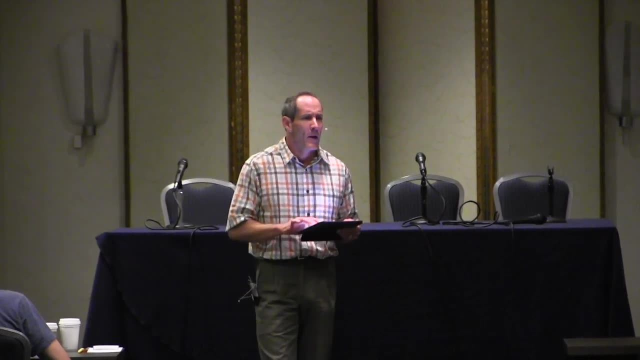 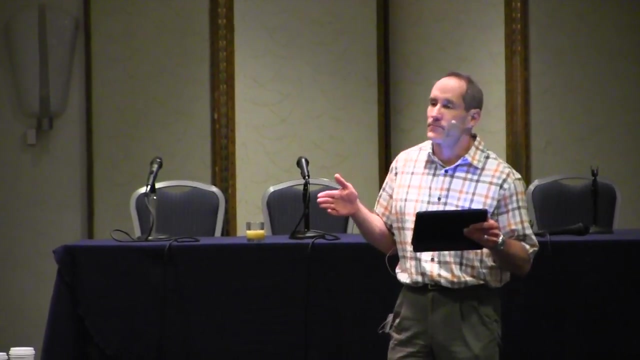 And that's pretty common. There are a lot of births Out there. I think my hospital births Something like 5000 kids a year, So you're going to get one or two Who has this. The typical presentation Is that the kid is born well. 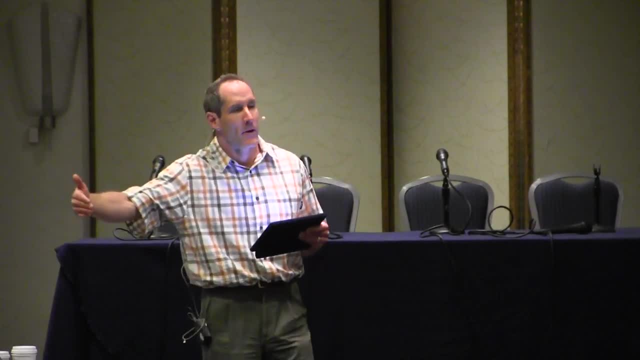 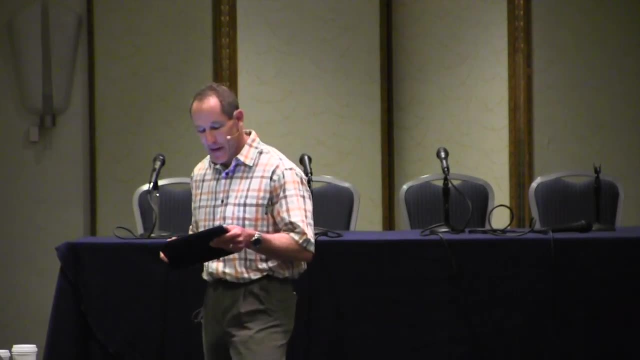 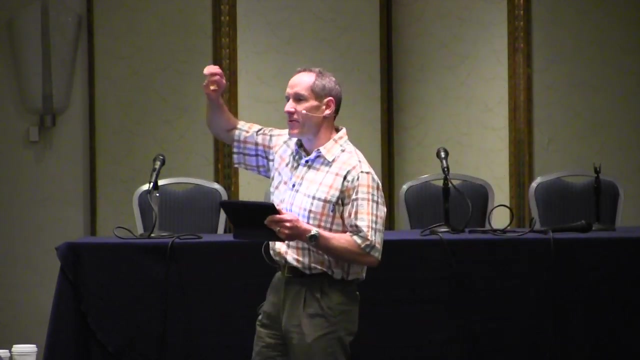 And then decompensates, Often within days, But it can be a little bit longer Down the pike too, And I think the best way to think about Inborn errors of metabolism Is That you start with A energy source. Which is essentially protein, And typically You're supposed to convert protein Into energy And An inborn error of metabolism Screws that up. So you start with protein And you don't end up with energy. Rather, you end up with a toxic metabolite. 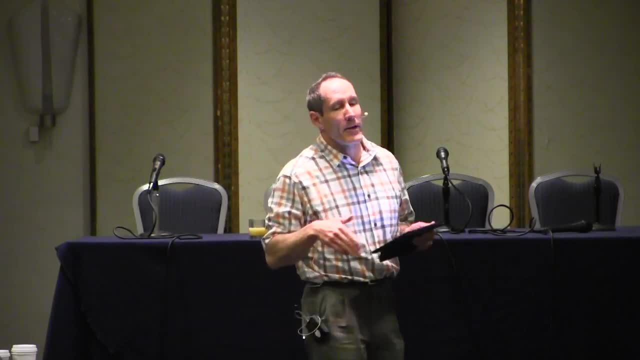 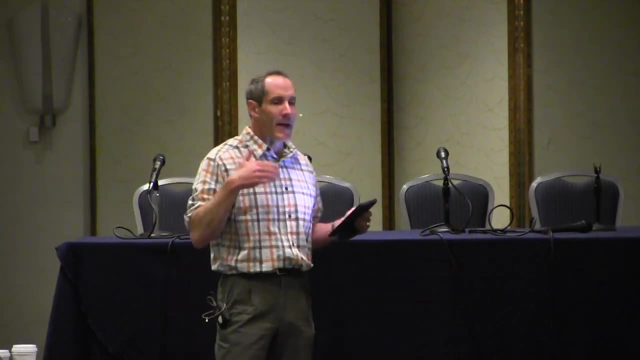 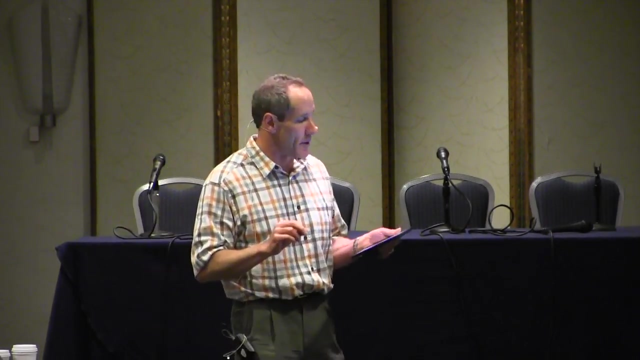 And so You get these kids who are presenting Typically Disease. So they often present neurologically And that can be lethargy Or altered mentation. Of course A four day old with altered mentation Might be a little hard to sort out. 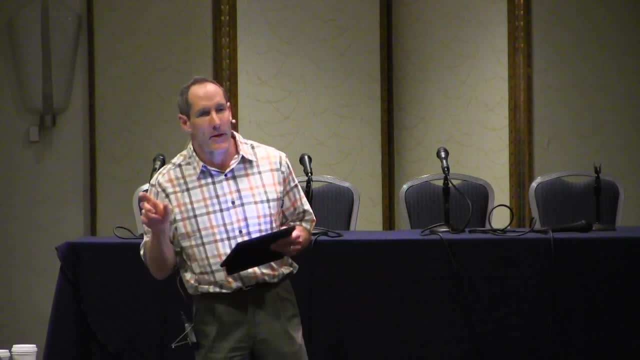 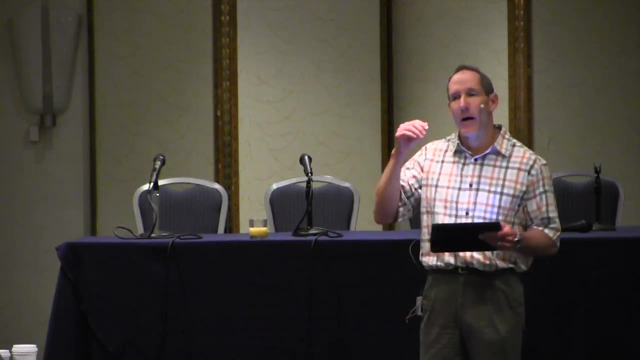 But you get a neurologic presentation often times. You get a GI presentation And you get a combination Often times. So It can present a lot like sepsis, That you get a kid who doesn't look good. They're sort of floppy. 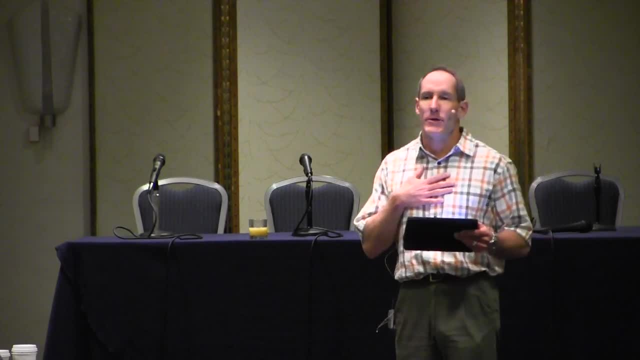 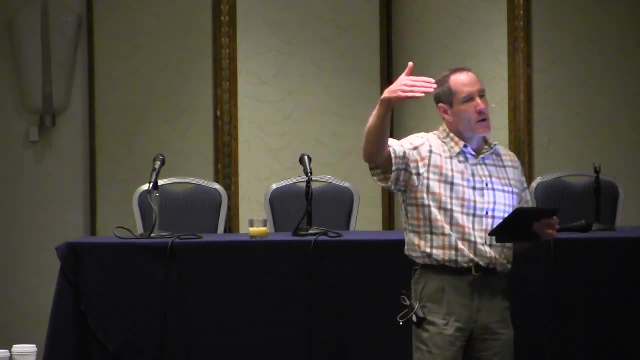 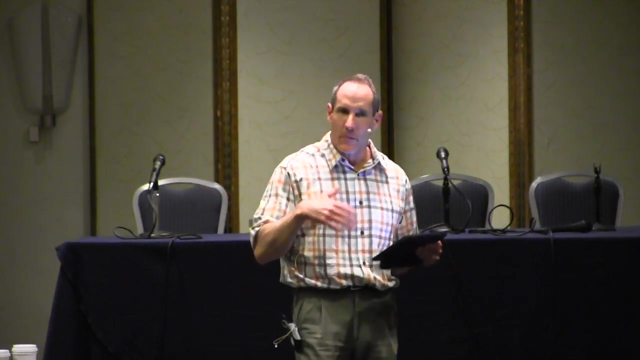 They're allergic, Maybe vomiting, And I think our knee jerk would be to say Sepsis And that's just fine. So go for it. Call it sepsis On your differential, But don't end your differential diagnosis there. So I think Anybody who sees a really sick Four day old, Seven day old Is going to think I'm going to give antibiotics And that's all great. But don't stop your thinking there. So if there was one test, 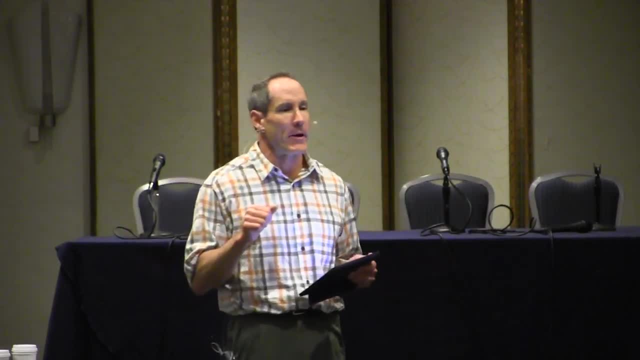 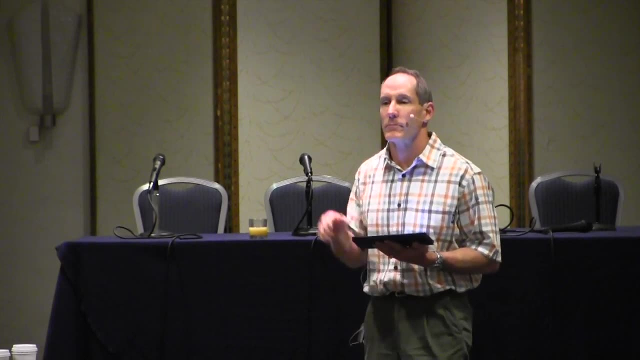 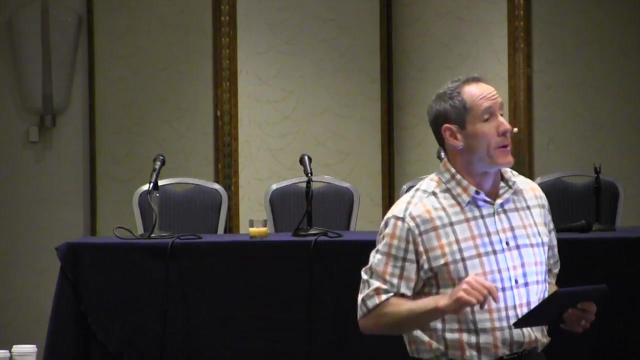 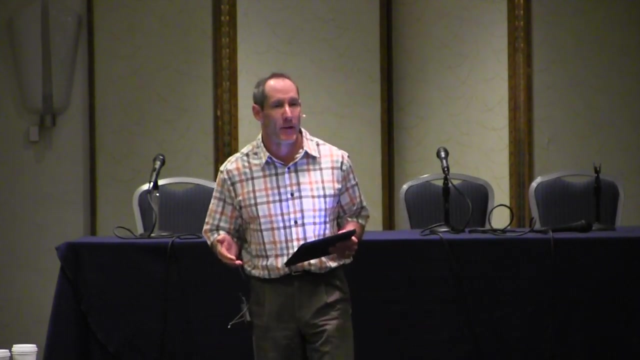 That you had to send To check for an inborn error of metabolism. What would the test be? One blood test. What Ammonia? Yes, So ammonia is your friend in this That we would normally think about sending, But ammonia levels. 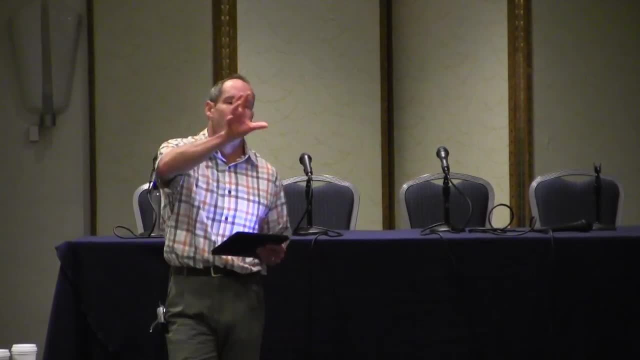 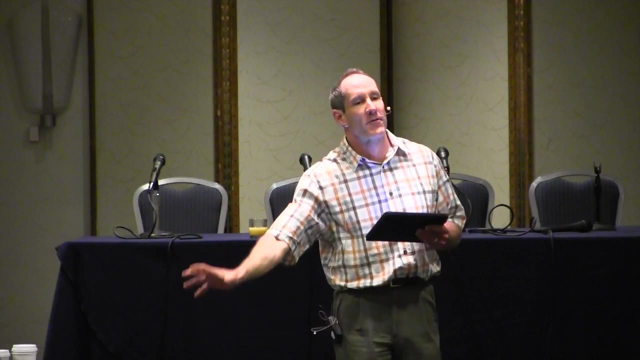 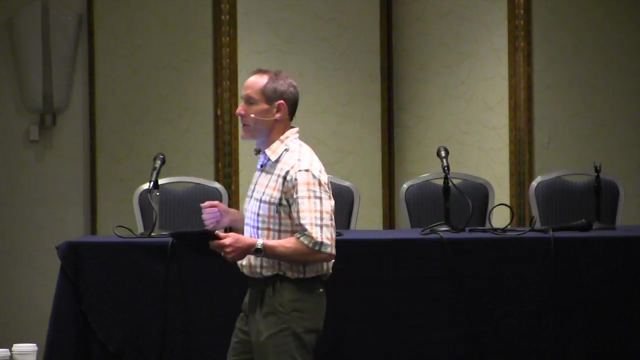 Can be markedly high. And this gets back to the. You got your protein That's not being metabolized And one of the toxic Metabolic effects Is you get a high ammonia build up. Now a sick kid, You can have a reasonably high ammonia build up as well. 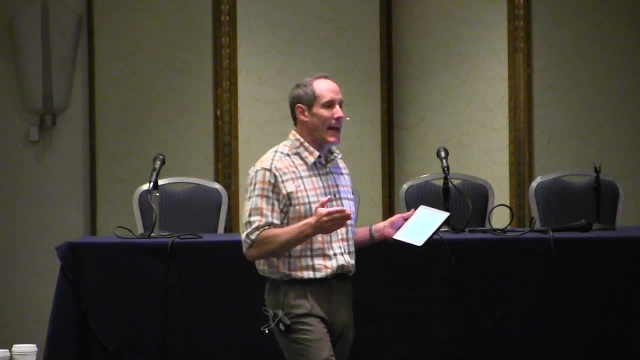 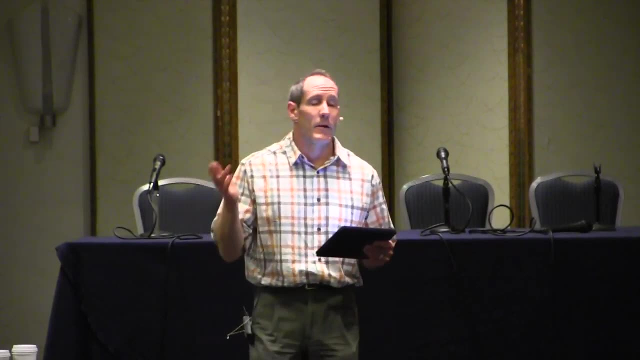 They talk about A cut off here of about 180.. So when you're seeing ammonia 180 or higher In that range, Start thinking inborn error of metabolism. But you've already been thinking it Because you sent the ammonia. 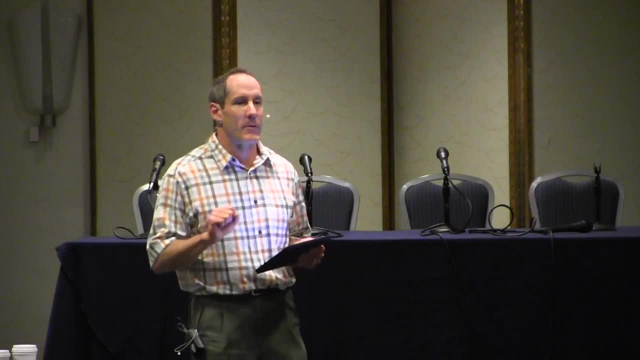 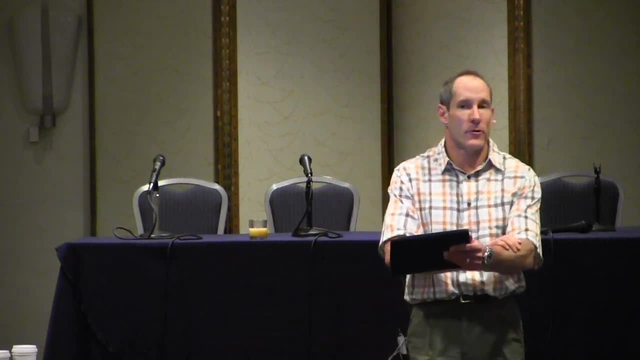 You weren't going to send the ammonia If you weren't thinking inborn errors of metabolism. Now, supposedly, You're supposed to send Either an arterial sample Or try not to put The tourniquet on the kid for too long. Because that in itself can build up ammonia In my ED. I'm just happy to get blood Out of a four day old. So I think you do the best you can, But just beware If your nurses or you Are working that kid's arm. 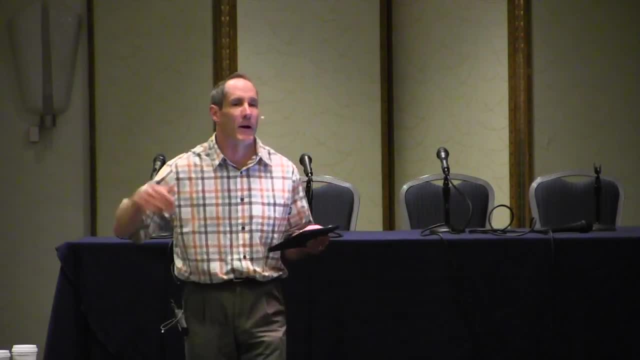 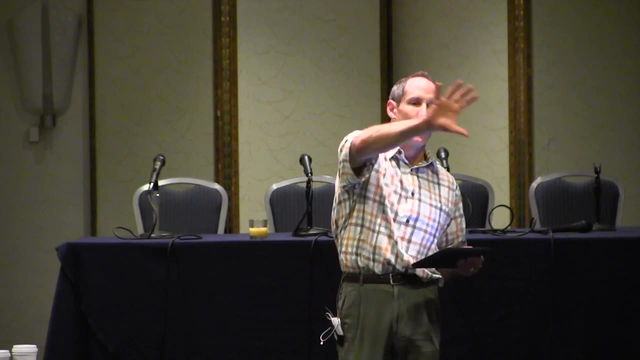 For 20 minutes With a tourniquet on it. That could be a false positive ammonia level. So how do you manage this? So we talked about You've got your protein That's not being properly metabolized. So the first thing you do 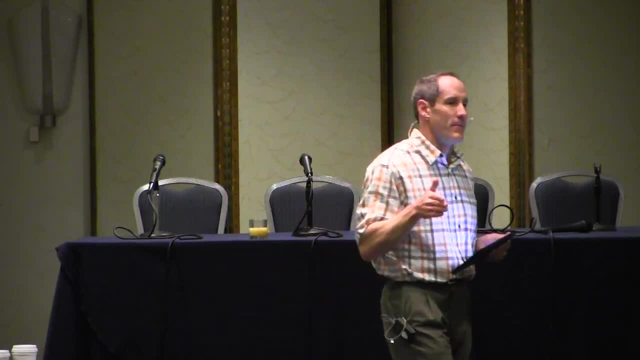 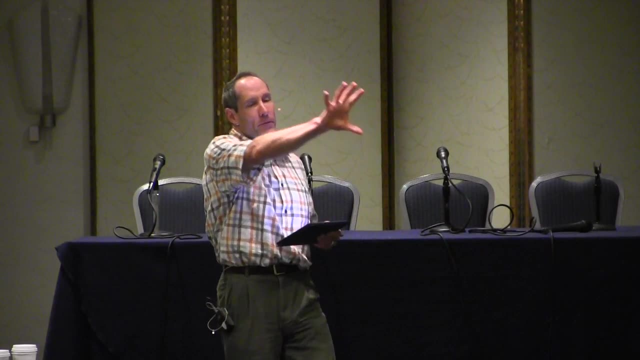 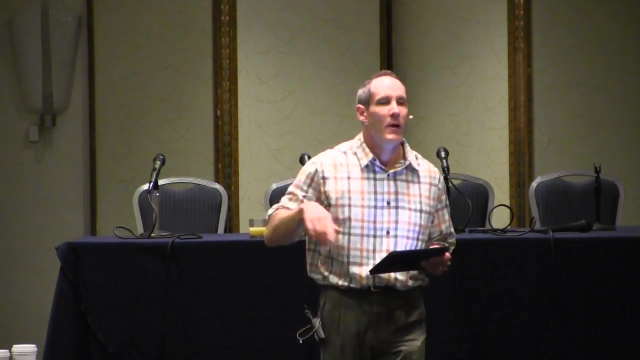 Is: stop your input Into this toxic system. You stop feeding the kid, So you make the kid NPO And then, as we talked about, The protein Turns into energy And you can't get that Through the kid's own mechanisms. 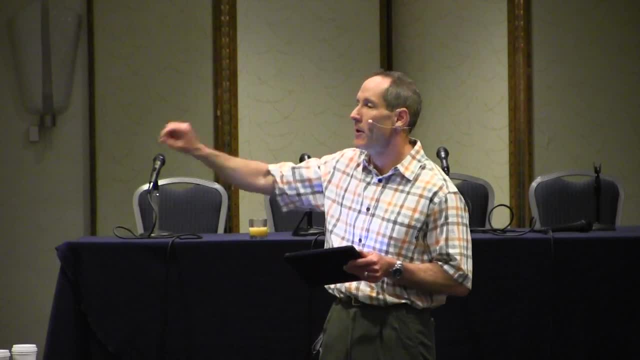 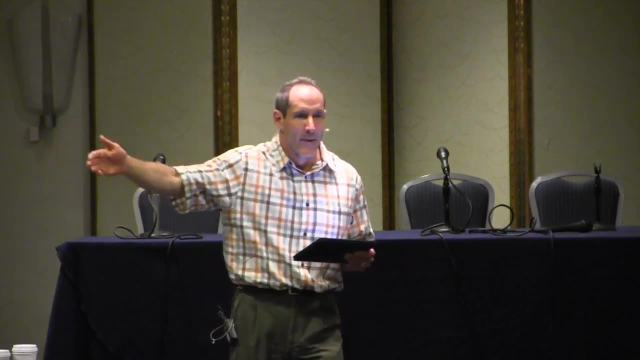 So you've got to supply the kid With his or her own source of energy, Meaning you give IV glucose. So you make the kid NPO, You give IV glucose And then You probably are going to call your consultant. So there are other things. 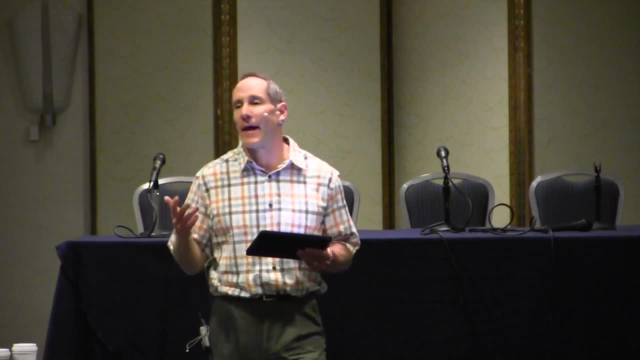 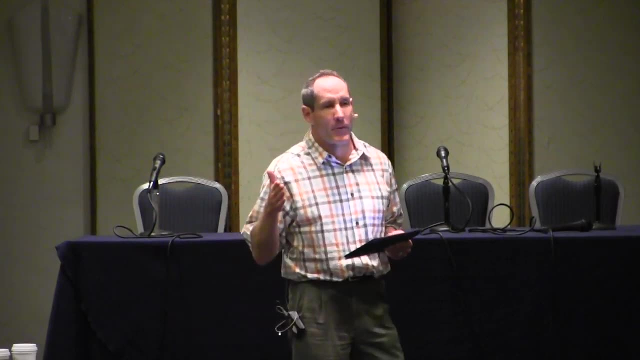 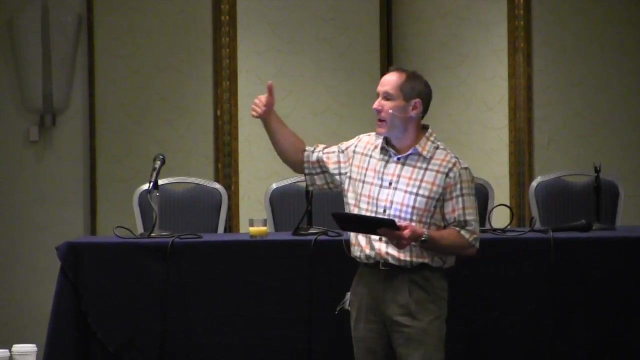 You can do, You can give other scavengers Of toxic metabolites. But I think if In the ED We just take a simplified approach, That you think about it, You order your ammonia, You make the kid NPO And you give IV glucose. 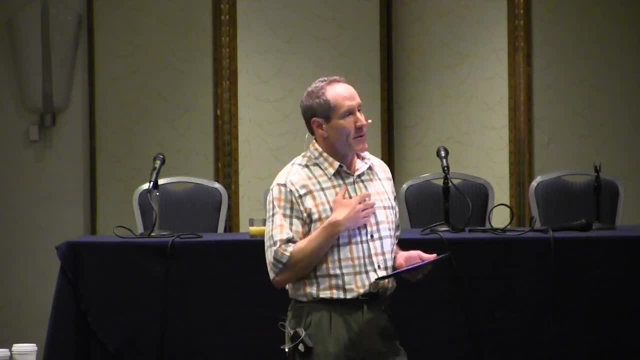 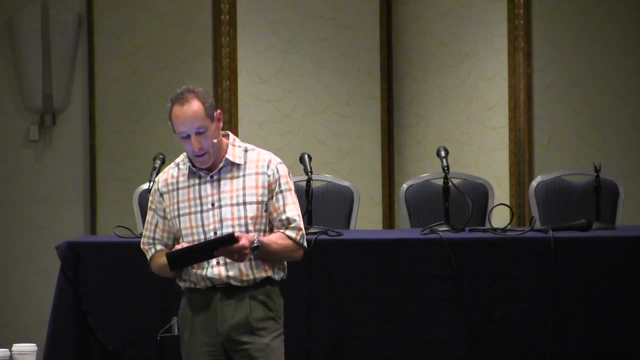 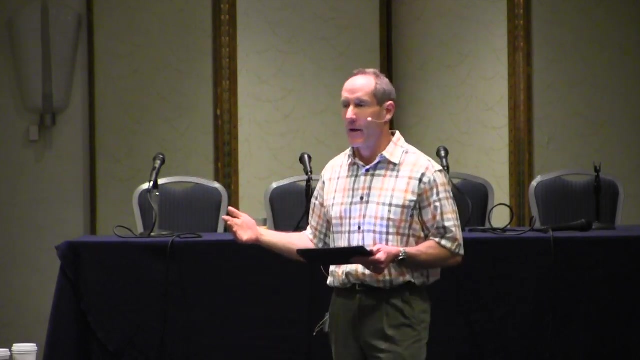 You've done a great job. Now bear in mind- And I didn't really appreciate this- That these are really sick kids And some series have reported A mortality rate Of 50%. So You can do everything right And these kids die anyway. 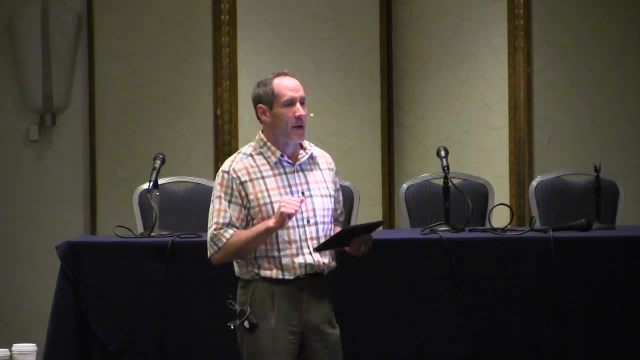 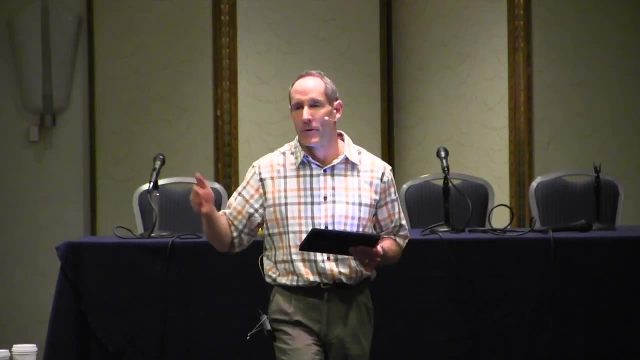 So it is rather sobering That these kids can get this sick. So just be aware of that And at the end of the day, If you have one of these cases, You did what you could And the kid died. That is often the outcome. 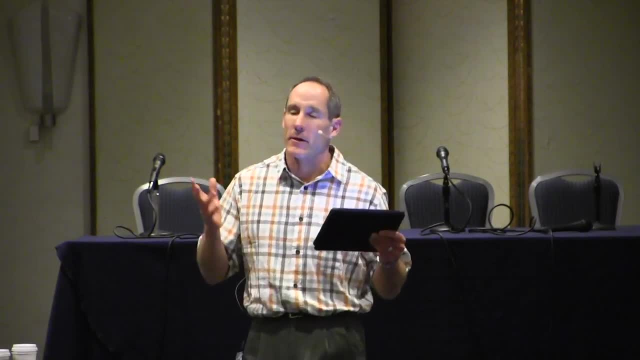 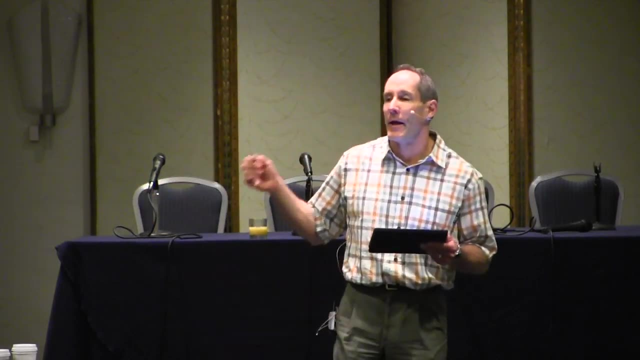 So one other thing I'll say About inborn errors of metabolism. If you ever see a seizing baby And you can't stop the seizure, That is one of the presentations of these And that is a Paradoxine deficiency. So you can give paradoxine. 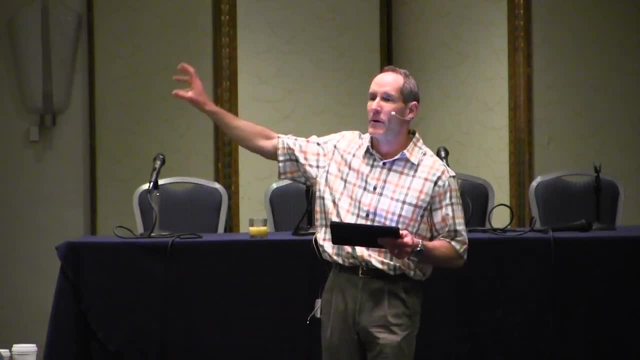 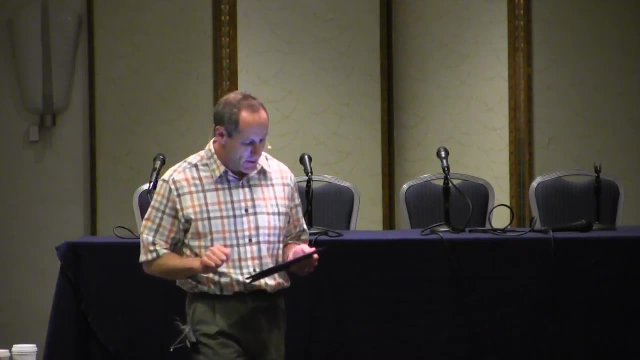 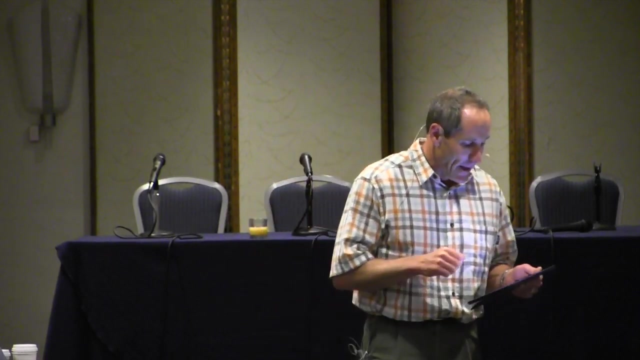 And that can treat the seizure. So again: seizure, Little baby, Think paradoxine. So final summary, Key points and recommendations: Kawasaki disease, And I didn't mention it's not Kawasaki's disease, It's Kawasaki disease, It's a. 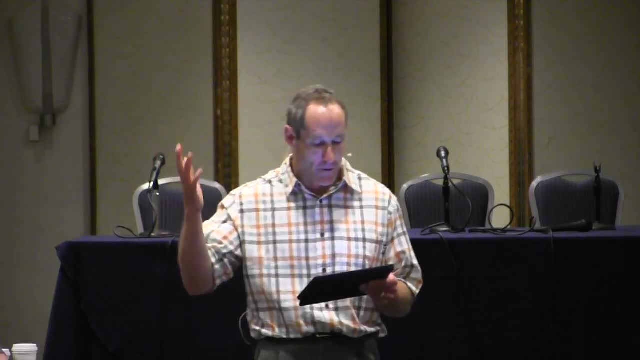 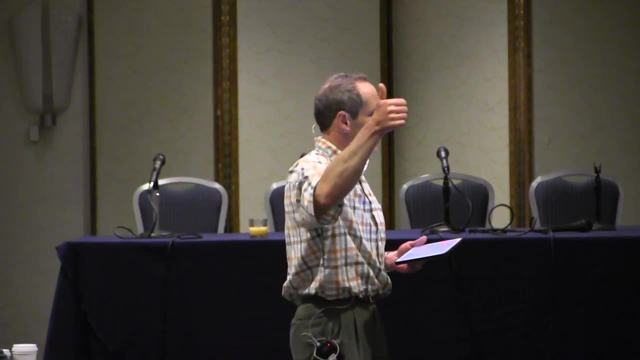 Inflammatory process. It's a vasculitis. But I never really understood what a vasculitis was, So we didn't focus on that. Those are the five criteria. You've got the five days of fever-ish. You've got the lips.